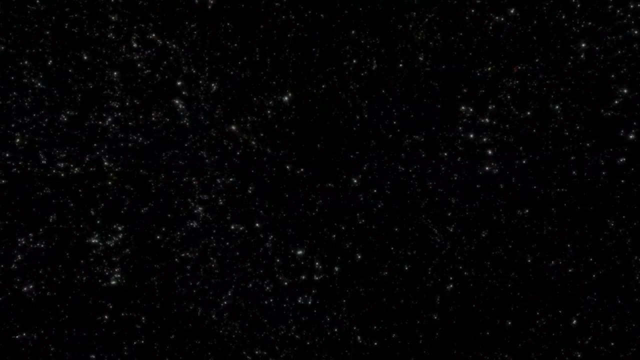 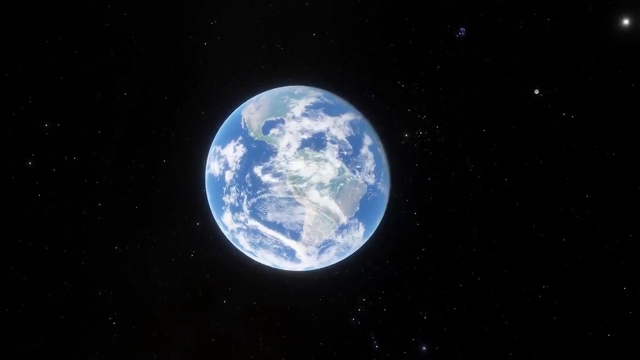 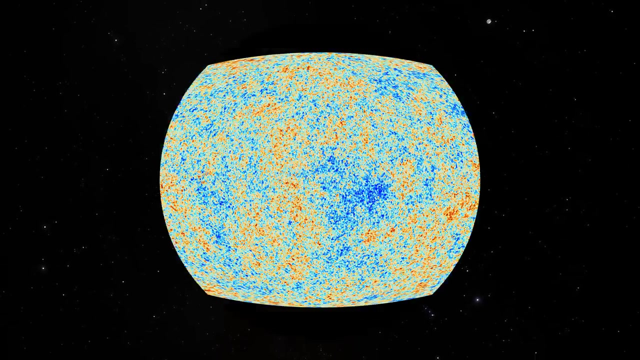 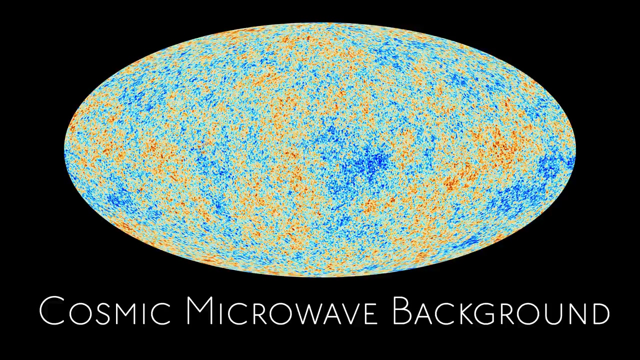 This static which sounds something like what you're hearing right now, is a microwave band low-pitched humming emanating from the ground, And if we map this noise with sensitive enough equipment, then it gives us the oldest map in the universe- the Cosmic Microwave Background, aka the Afterglow of the Big Bang. 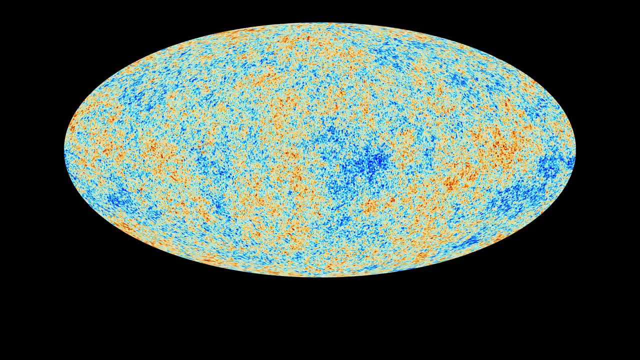 This map provides us a clear window into the early universe and is the most deep and complete collection of cosmic knowledge that we have. This map provides us a clear window into the early universe and is the most deep and complete collection of cosmic knowledge that we have. 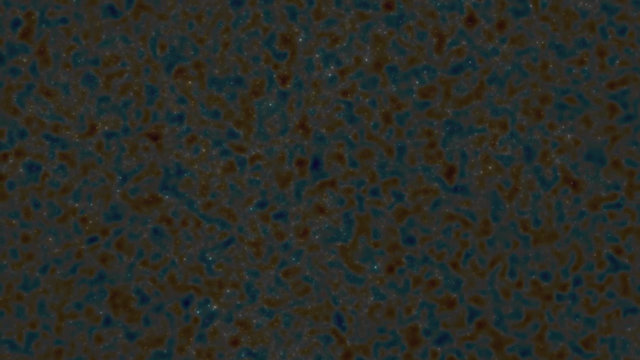 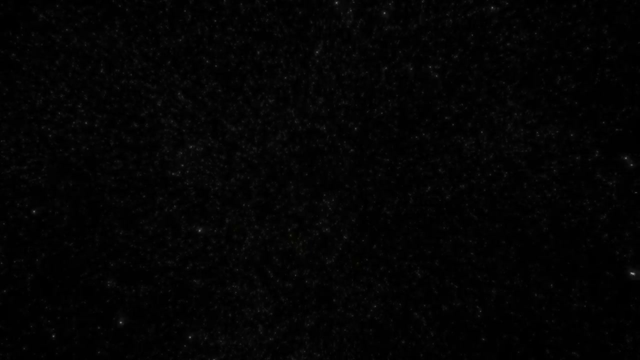 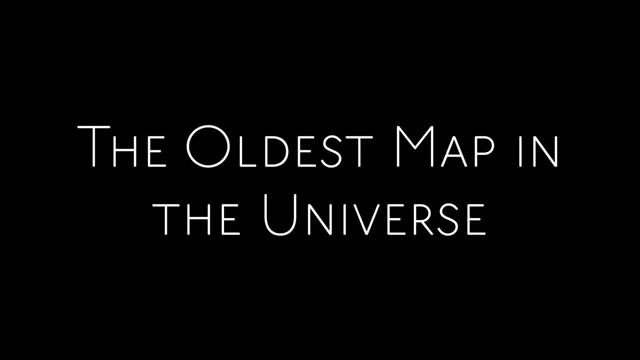 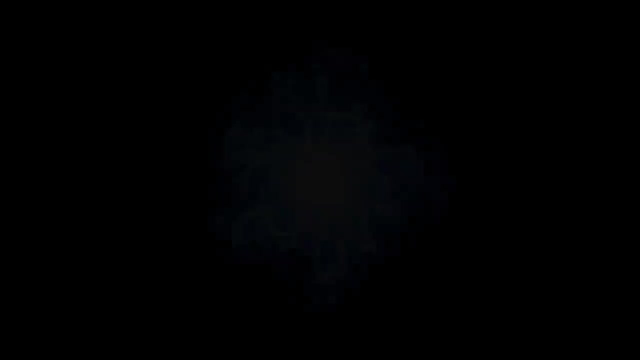 It allows us to deduce large amounts of information about our universe today and provides crucial evidence for the Big Bang as we understand it. That's where our story begins today- The Big Bang All the way back near the beginning of time. The Cosmic Microwave Background is fundamentally linked to the Big Bang. It is the relic radiation. 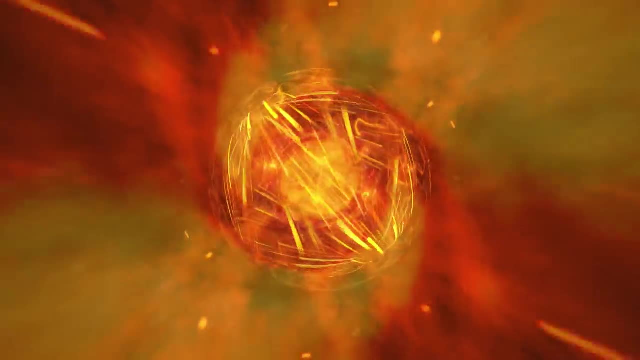 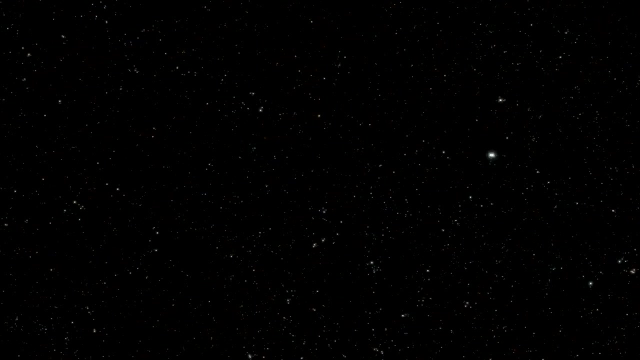 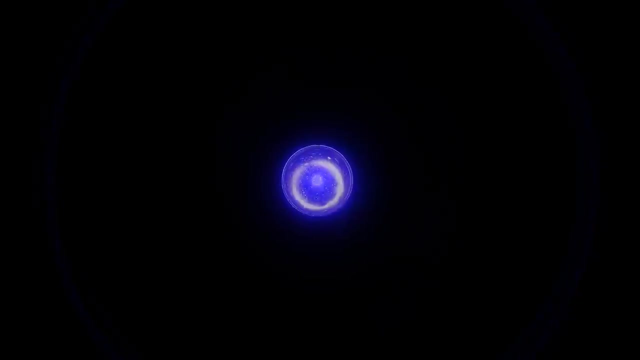 from the final stages of the early universe, before it became the vast dark expanse that we know it as today. The Big Bang theory holds that the universe began from a microscopic volume of unimaginable heat and density little under 14 billion years ago- a volume that 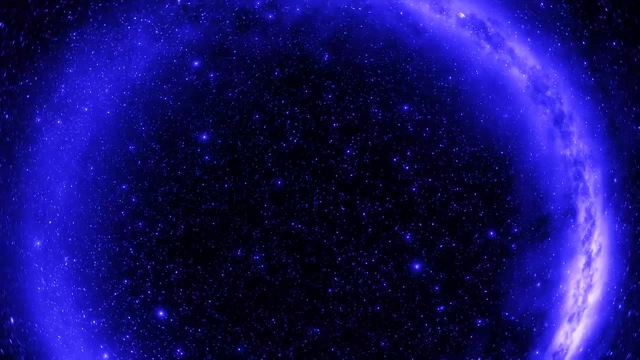 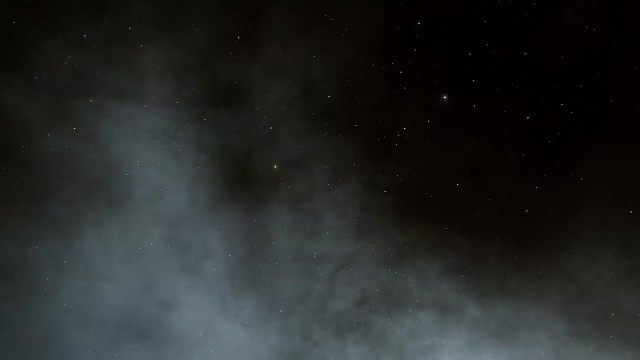 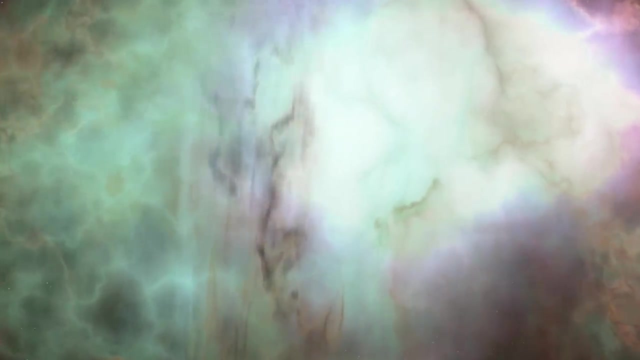 has been expanding ever since. In reality, the use of the word bang can be a little misleading- it suggests that a single explosion event at time zero gave rise to the universe. In actual fact, it would be more reasonable to say that the universe was a giant continuous explosion up until around 380,000. 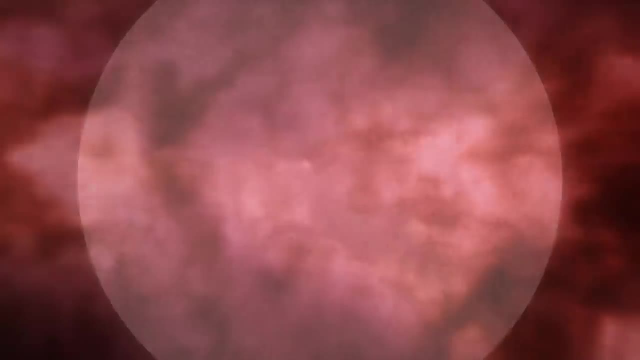 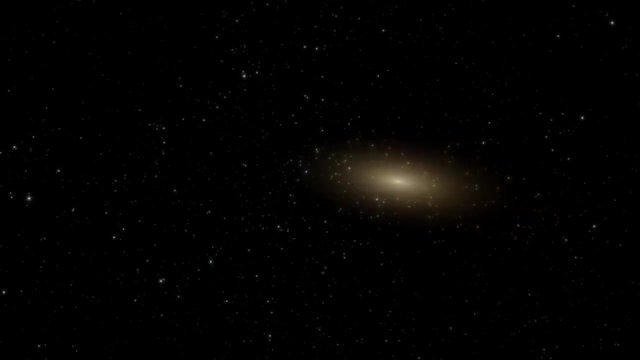 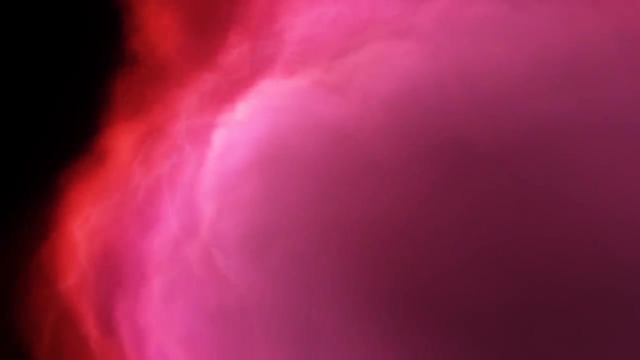 years after it was born. Before that, it was considerably smaller and its contents- all the galaxies and matter in the universe today- were crushed into an area millions of times smaller than the space they currently occupy. Temperatures sat well above 100 million kelvin- so hot that 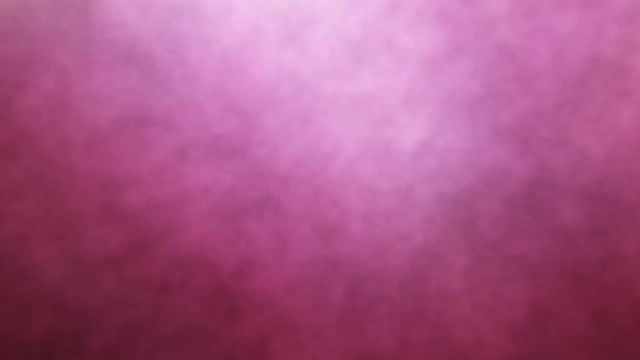 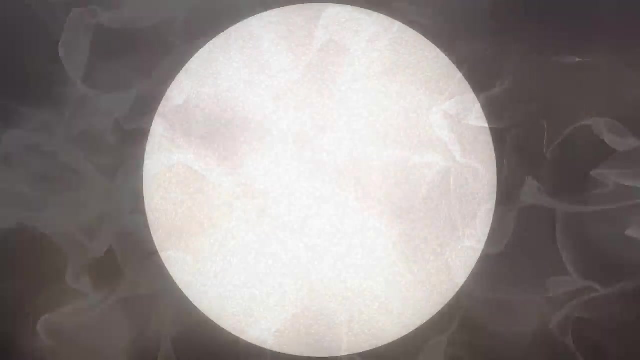 light and matter could not be separated. locked together in an ultra-energised, white-hot soup which flooded all of space As the universe expanded in its early years, these contents spread out and cooled Particles formed inside of the universe and particles formed inside. 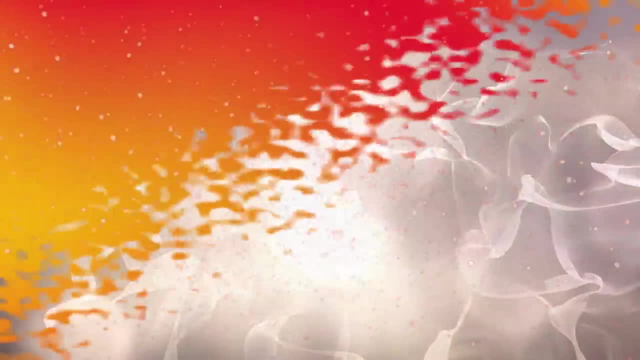 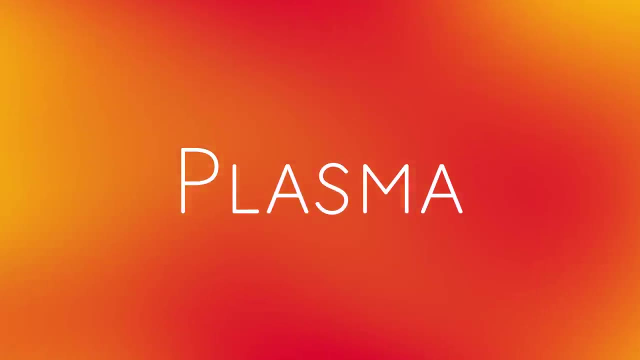 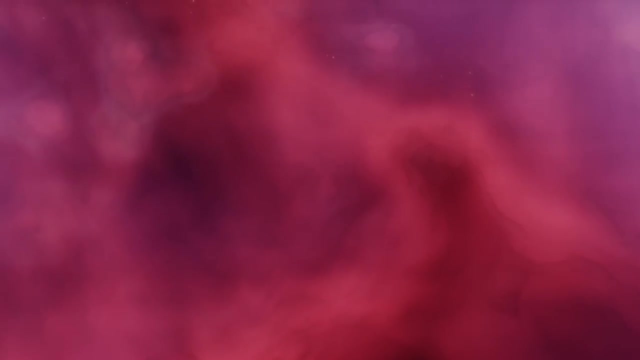 of it, and the white-hot soup evolved into an opaque orange fog consisting of free-roaming electrons and exposed hydrogen nuclei- known as a plasma. Within this plasma, the temperature was still far too hot to allow subatomic particles to latch onto one another and form atoms, and instead 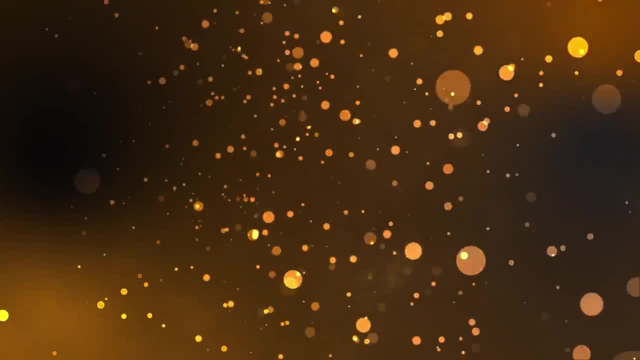 they darted across space randomly and chaotically, coming together and breaking up. Localised interactions were occurring within the plasma as the galaxy's atmosphere changed and the galaxy's atmosphere changed, as the galaxy's atmosphere changed and the galaxy's atmosphere. 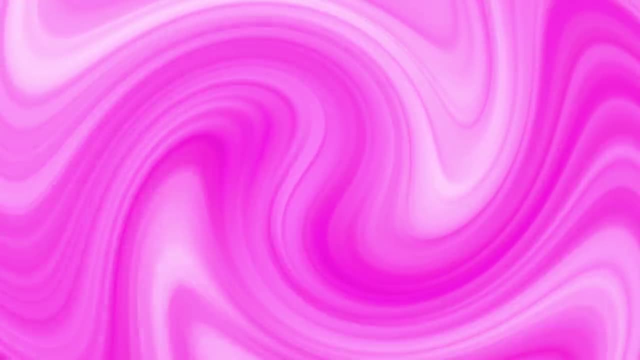 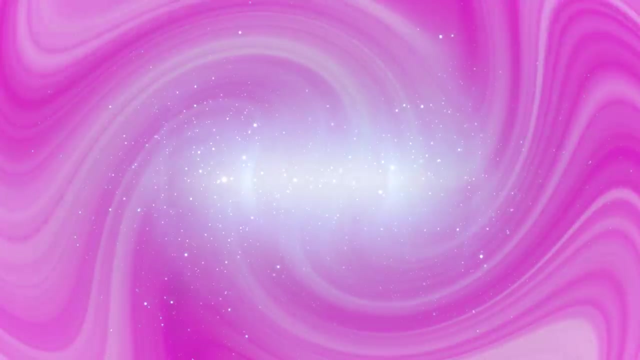 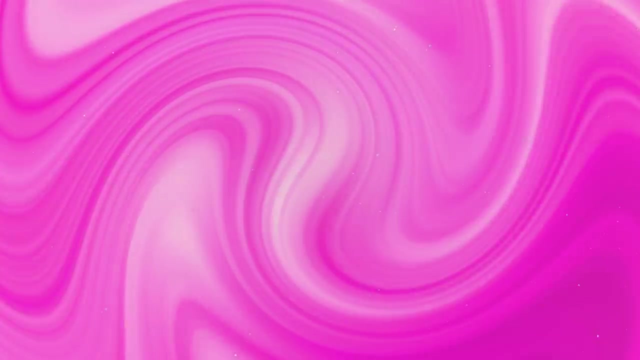 changed and the gravitational pulling force of its matter tussled with the outward radiation pressure of its light. The colliding and dispersing of concentrations of matter generated acoustic sound waves which flowed outwards, tracing oscillatory patterns within the plasma contents which added a degree of randomness to its near uniformity. 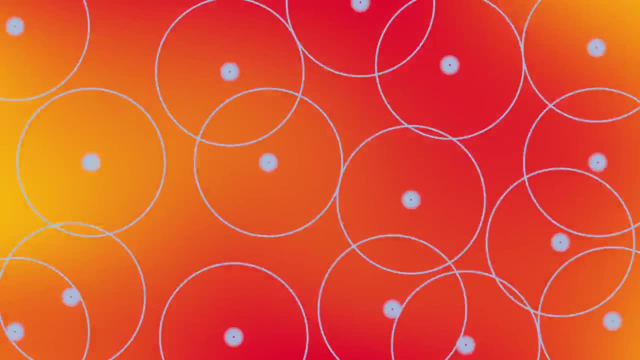 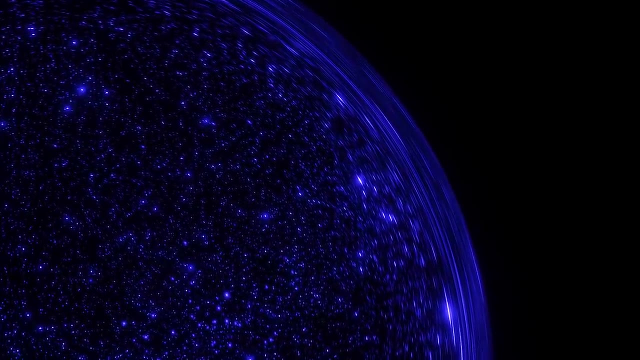 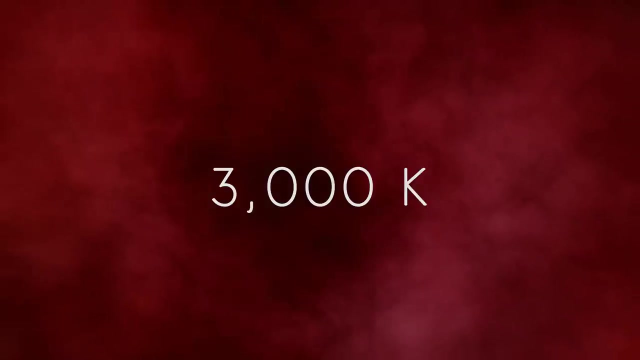 And then, at around 379,000 years after the universe was born, it expanded to around 1100 of its current size. Its interior temperature fell to around 3000 kelvin. Suddenly, it was no longer hot enough to maintain the universe's plasma state, And so, instead of zipping around free-roaming, 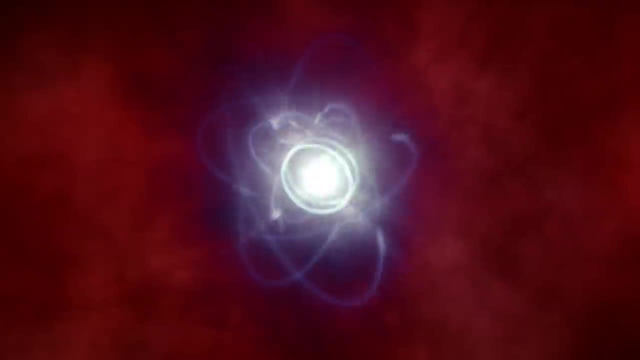 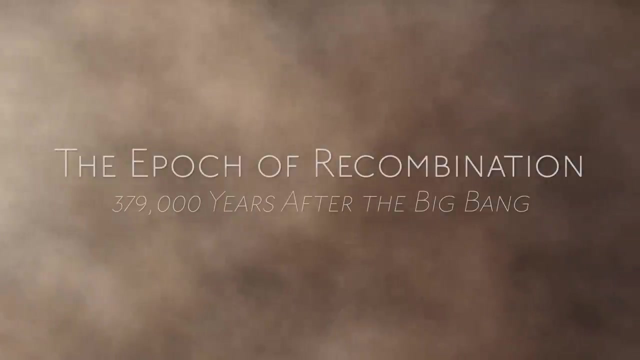 electrons began latching onto exposed atomic nuclei and could remain stable. The plasma was harvested all over the universe in an event known as the Epoch of Recombination- a process which created the universe's plasma. The Epoch of Recombination was a process which created the 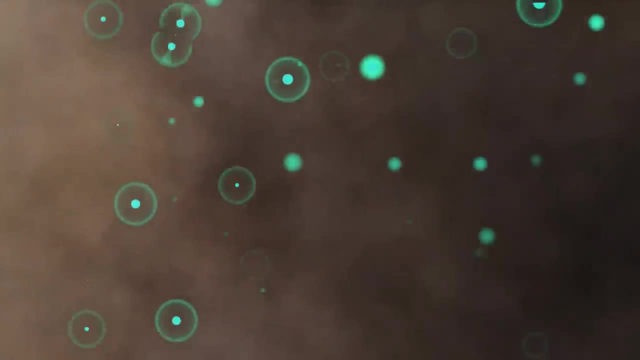 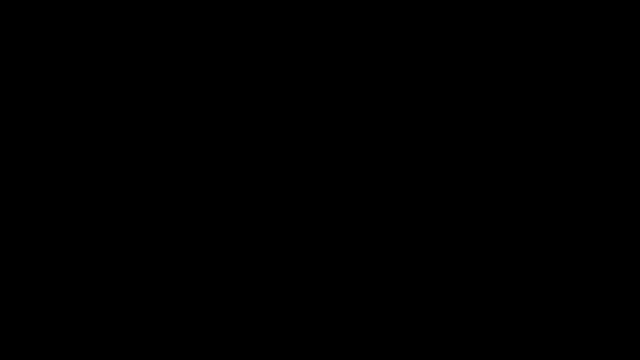 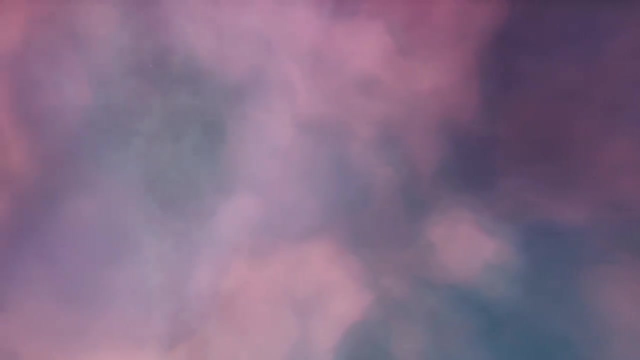 universe's plasma. The Epoch of Recombination was a process which created the universe's first neutral hydrogen atoms. Unlike within an ionised plasma, photons of light are barely affected by hitting neutral hydrogen, and so light could now travel freely and indefinitely around the universe. Matter and light decoupled from each other as photons were no longer being. 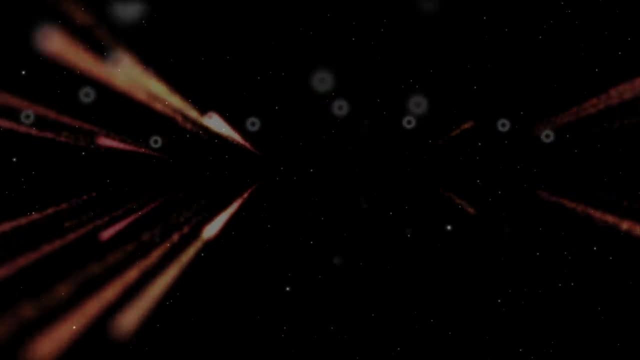 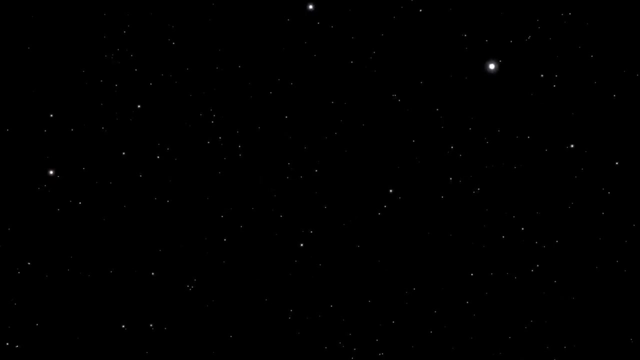 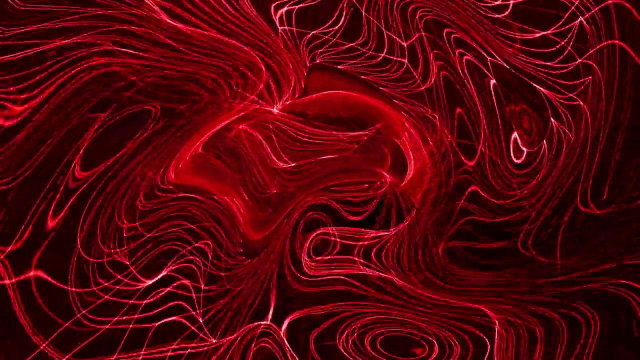 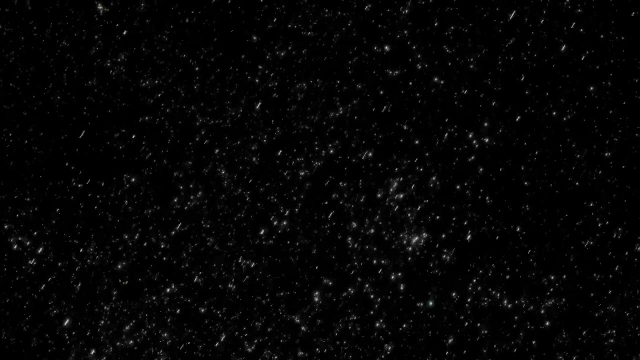 absorbed and the universe went from resembling an opaque orange fog to a transparent black void through which light could stream. During this transition event, the final acoustic wave patterns traced into the plasma by the baryonic acoustic oscillations were forever frozen into the arrangement of the universe's contents. Atoms formed along the framework laid by the 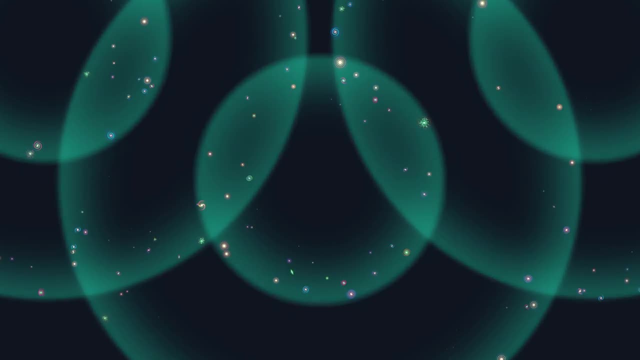 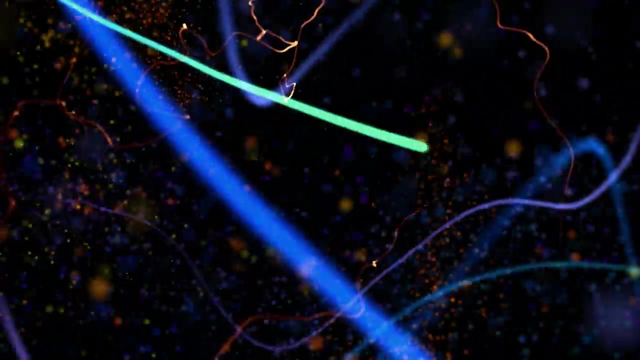 oscillatory patterns, creating denser areas where matter was in the process of coming together and sparser areas in which matter had been cleared out. The final photon, the Epoch of Recombination, was emitted by the energised plasma in its dying breaths, then scattered off of this arrangement. 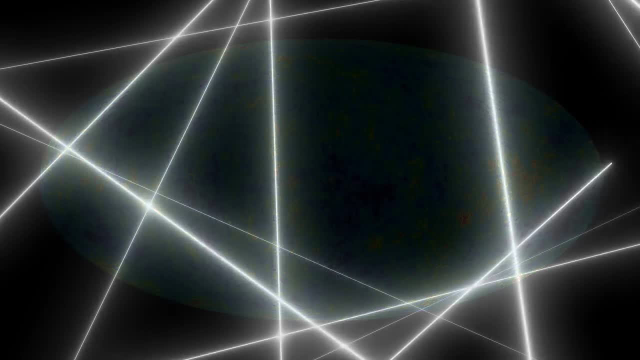 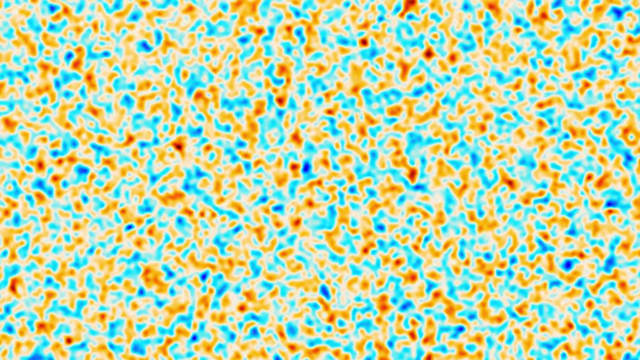 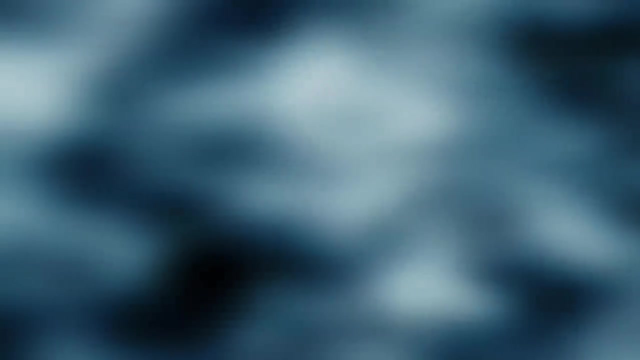 one last time before becoming free to shoot around the universe forevermore. That's what the CMB is: the final photons of light emitted from when this plasma turned to atoms, marking the end of the Big Bang. Therefore, the CMB is the oldest light in the universe that we. 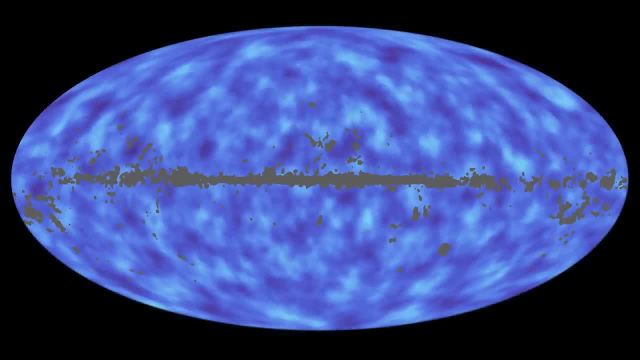 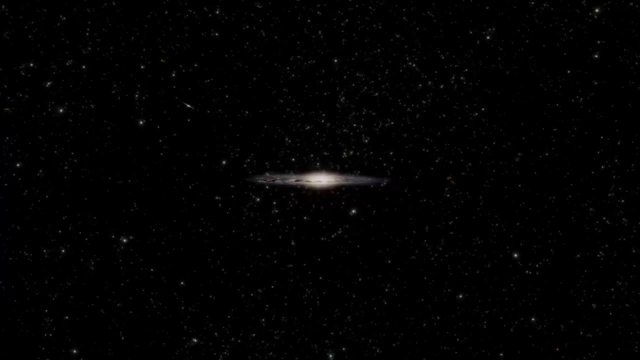 are able to see or detect, But these aren't photons of light. they are photons of light. The universe has been expanding for almost 14 billion years ever since, and all the while its growth has been stretching out waves of travelling light in space. 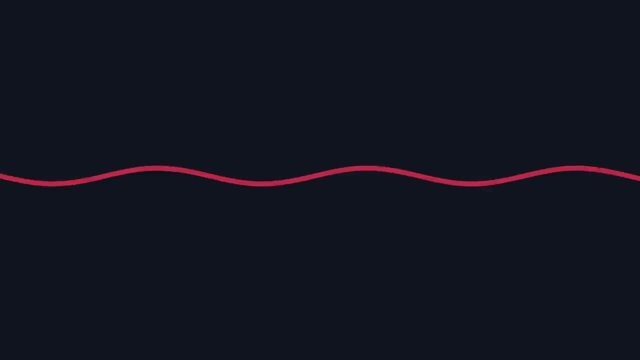 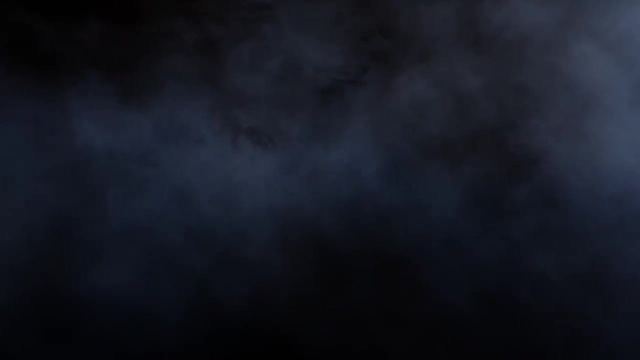 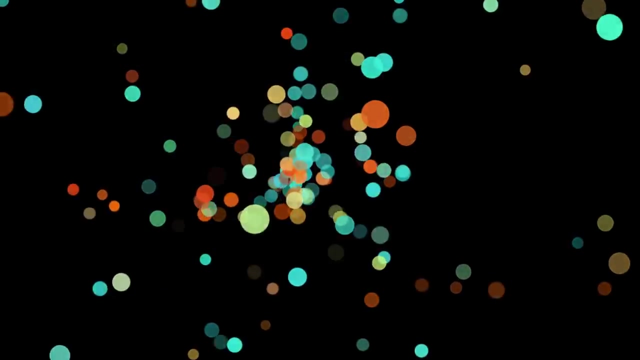 reducing their photon energy and shifting them through the electromagnetic spectrum. Today, the CMB's photon energy has been reduced by an average factor of 1090.. Before long, these photons were redshifted out of the optical spectrum and into the infrared spectrum, and then into the microwave spectrum. 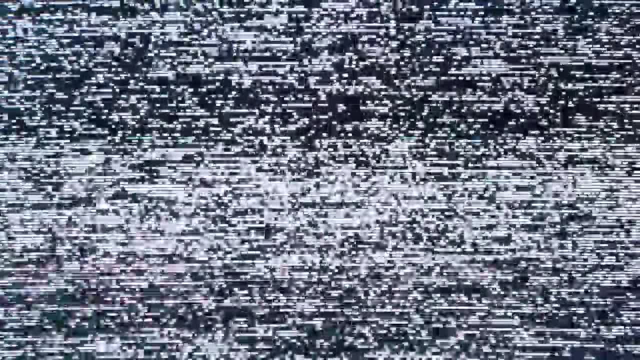 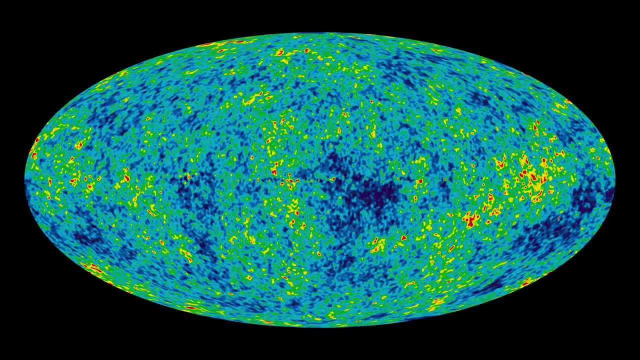 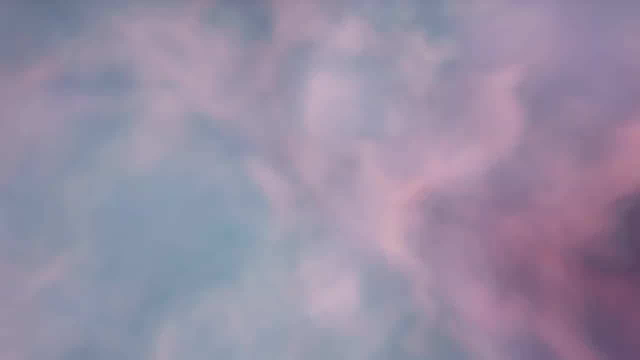 where we can now detect them as this faint humming between the airwaves. Thus, if we map this ancient cold light precisely enough, we can analyse the universe as it was during the moment of recombination, only 379,000 years after the birth of the universe- the furthest back in time it is possible to look. 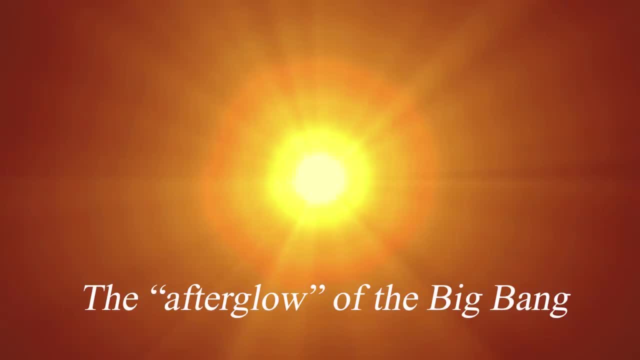 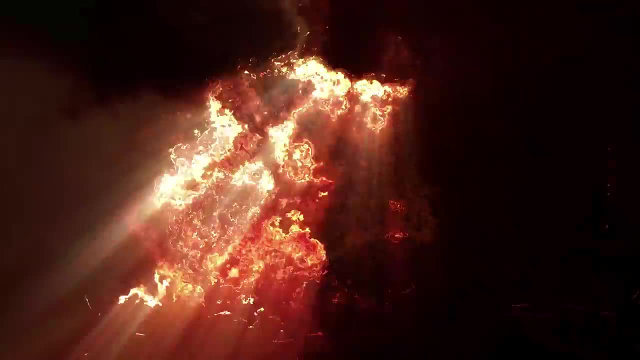 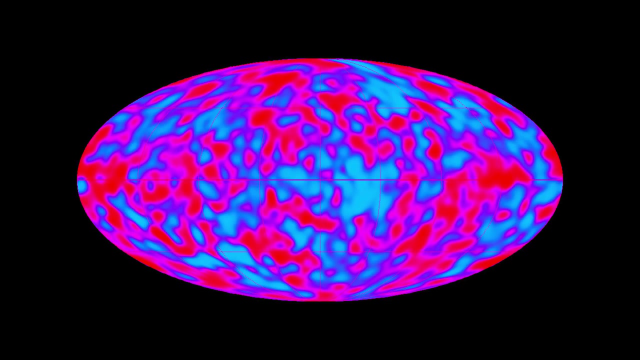 This is why the CMB is commonly referred to as the Afterglow of the Big Bang. It is relic radiation from the final seconds of the universe's fiery initiation, and it yields an incredible wealth of information about the properties of our universe both then and 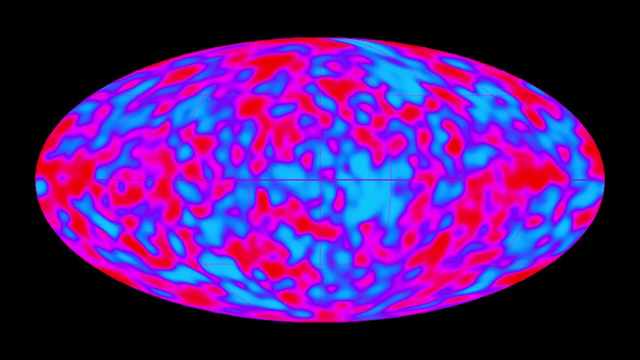 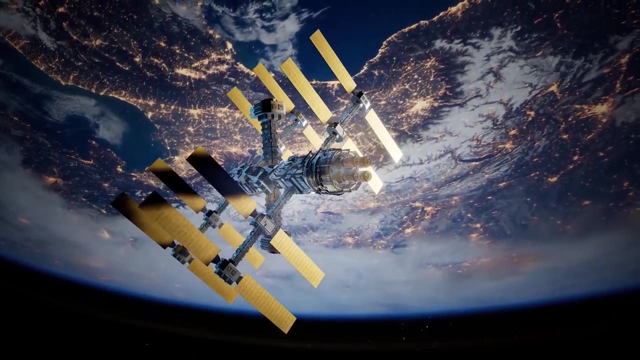 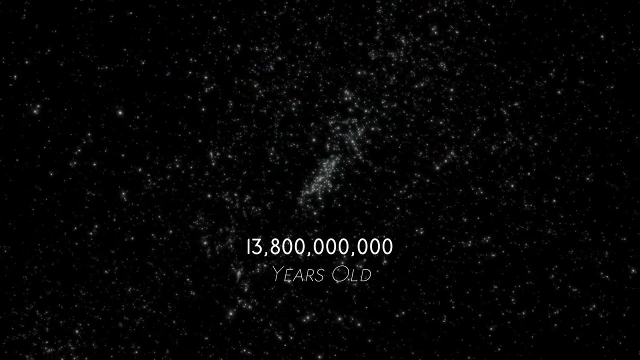 now. There are still many unknowns, and we are always striving for greater accuracy, But if nothing else, the CMB's existence effectively proves two things. The first is that the universe is around 13.8 billion years old, and the second is that it was much smaller and hotter early in its life. Two major postulations. 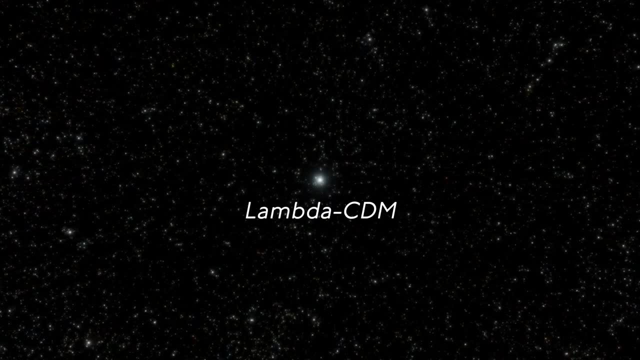 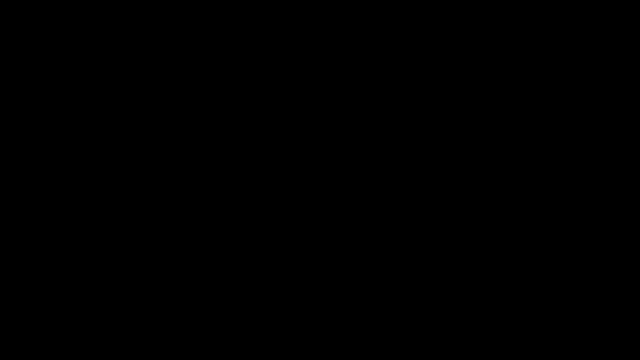 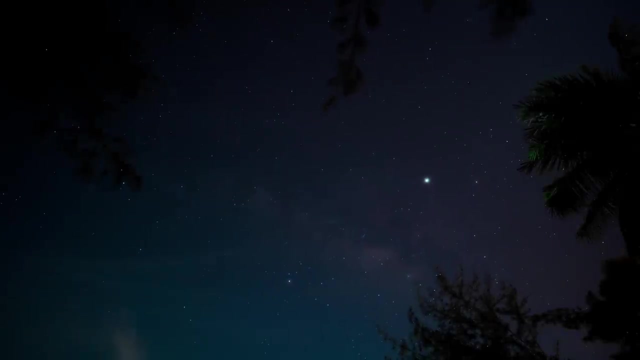 of the Lambda Cold Dark Matter model of cosmology- the standard model for astronomers and the theory you're most likely to find in the textbooks. This afterglow has been present in the sky for as long as humanity has existed, but we didn't discover it until the 1960s, when the advent of radio astronomy. 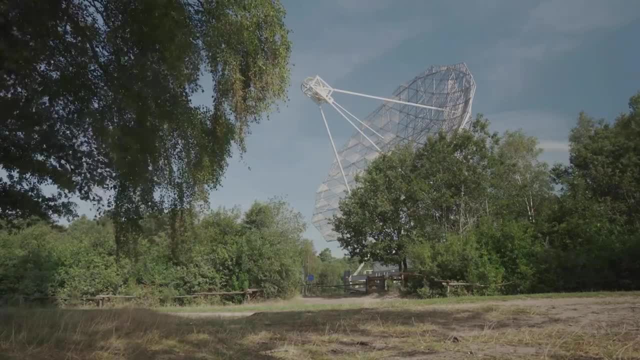 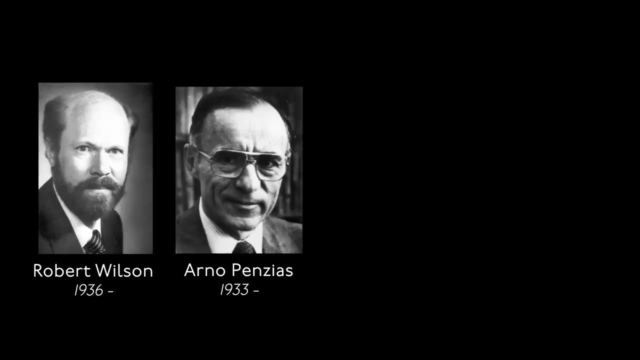 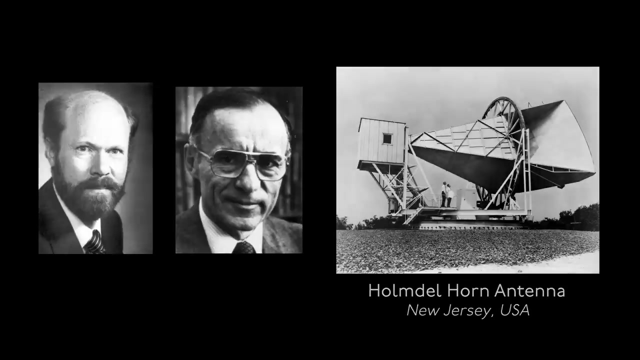 first allowed us to pick it up. On the 20th of May 1964, American astronomers Robert Wilson and Arno Penzias of Bell Telephone Laboratories were attempting to use the Holmdelhorn antenna in New Jersey to search for sources of static. so that they could improve the quality of telecommunications. What they found was that, no matter where they tuned their antenna, there was always a consistent excess temperature which could not be accounted for. In the words of Penzias himself, it wasn't until they had exhausted every other possible. 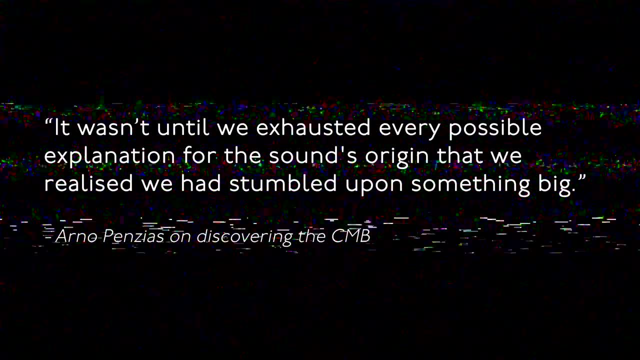 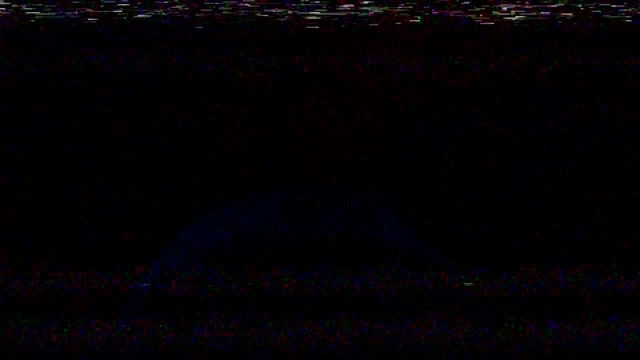 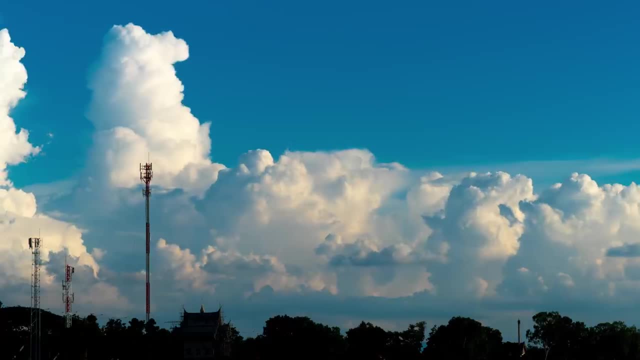 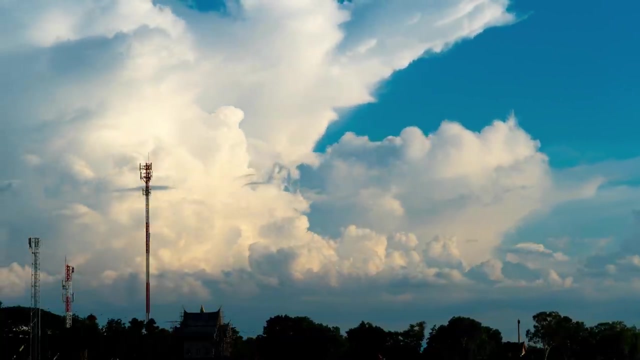 explanation for the sound's origin that they realised they had stumbled across something, And something big indeed. it was Arguably one of the most important and iconic scientific discoveries of all time. Initially, radio technology wasn't sensitive enough to detect any variations in this microwave humming. This is because the CMB has a nearly uniform 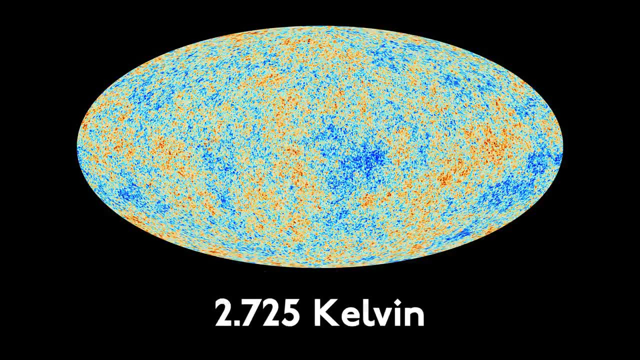 average temperature of 2.725 Kelvin, with variations of only one part per 100,000 or less. And so when we started our research, we found that the CMB had an average temperature of 2.725 Kelvin. And so, when we started our research, we found that the CMB had an average temperature of 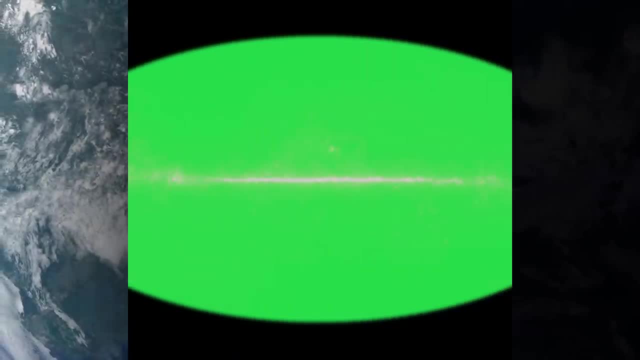 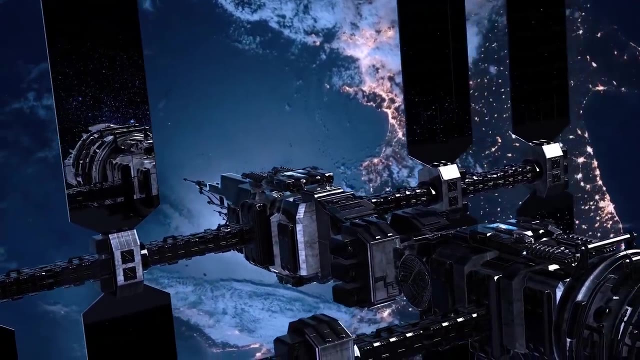 2.725 Kelvin, And so when we started our research, we found that the CMB had an average temperature of 2.725 Kelvin, And so when we started surveying the microwave sky, it seemed to be completely uniform. But we've spent over 60 years and more than a billion dollars refining and improving our 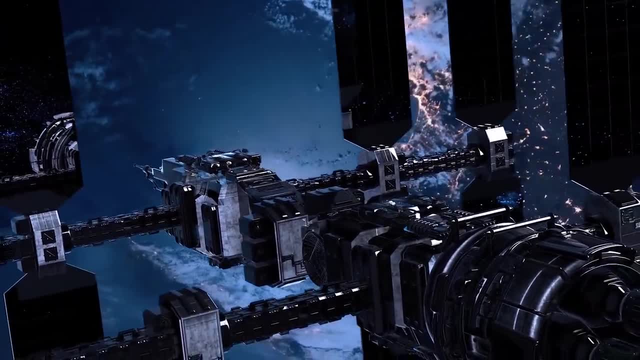 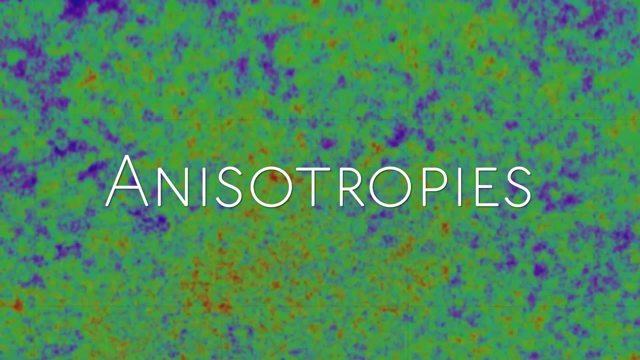 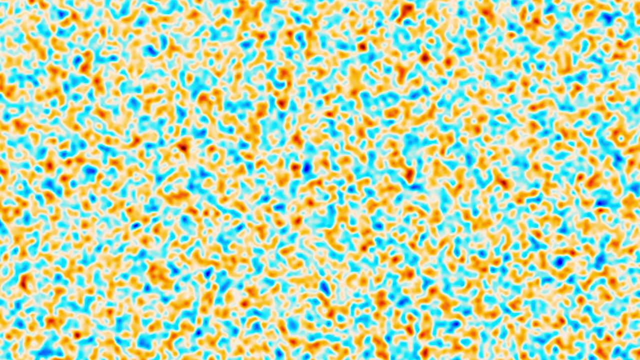 mapping technology revealing tiny temperature fluctuations on scales of a matter of microKelvin known as anisotropies. The CMB's anisotropies are its tiny treasure chests containing some of the most important information about the universe ever discovered. 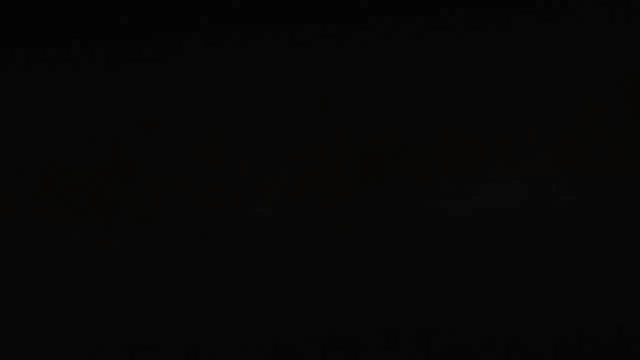 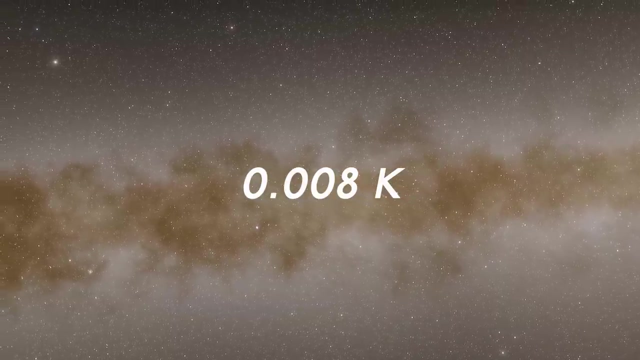 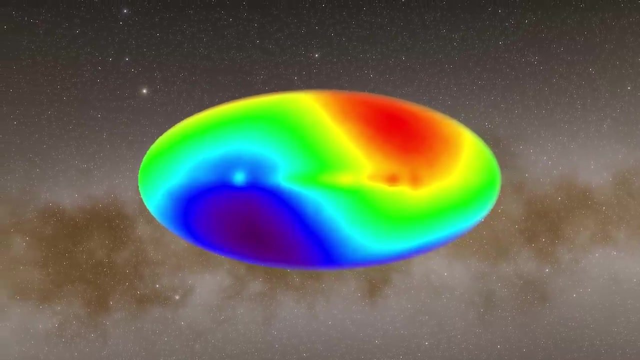 The first and largest anisotropy we found was a temperature change of around 0.008 Kelvin On this scale. the microwave sky appears to resemble a yin-yang symbol. However, this is not a result of the Big Bang, but rather a result of the Sun and the Milky Way galaxy moving. 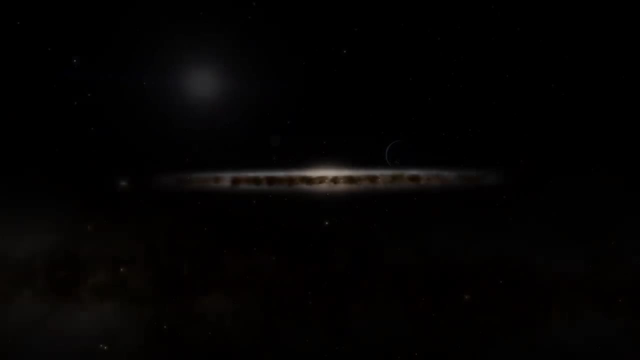 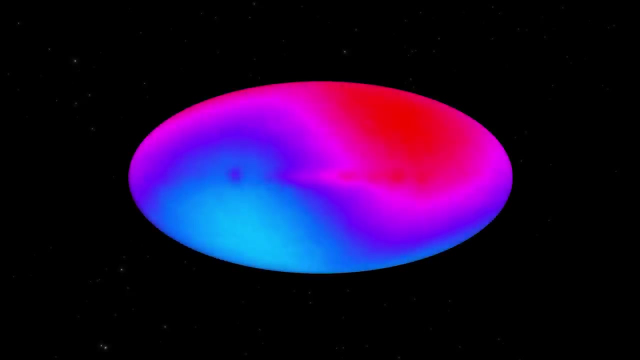 through space towards a series of galaxy clusters, known as the Great Attractor. This creates a temperature gradient in the microwave sky, which is known as the Great Attractor. This creates a sky from one side to the other, known as the Dipole Anisotropy. Once we'd smoothed that out, 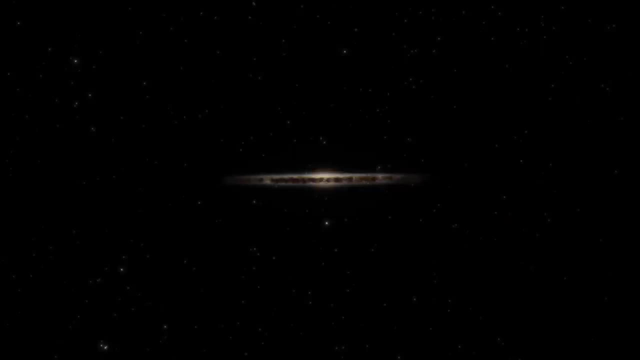 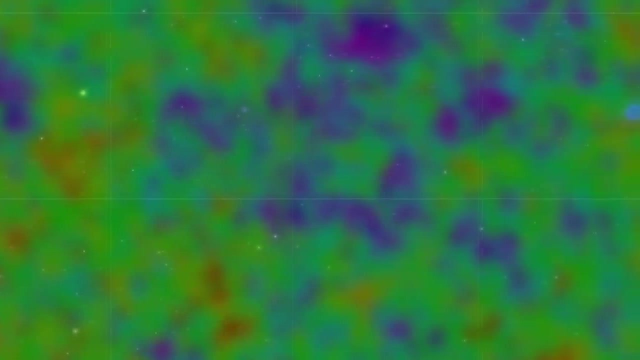 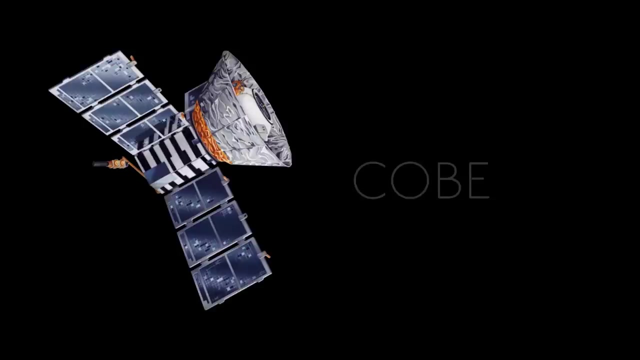 and accounted for the dipole. we had to get down to scales of around 30 times more precise before we were able to see any real differences. NASA's first big breakthrough contribution to this quest was the Cosmic Background Explorer, also known as COBE. It launched in 1989 and collected data up 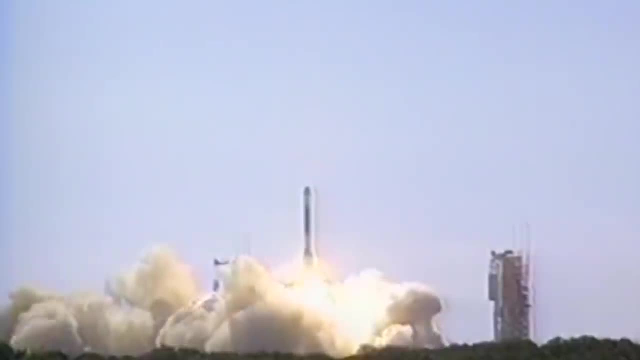 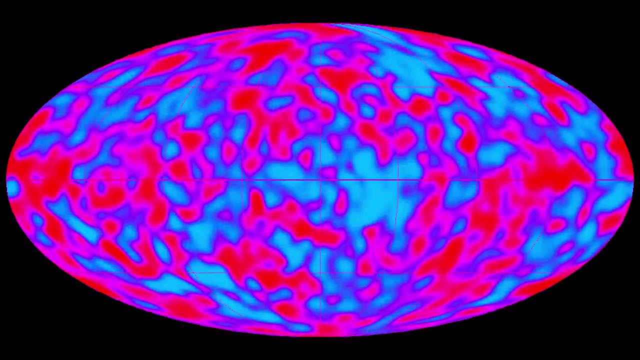 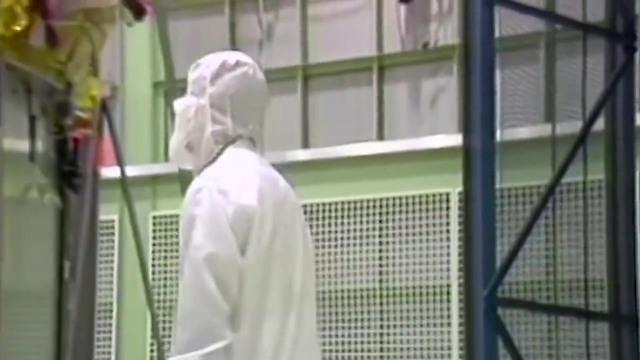 to 10 years ago. It built upon work from previous ground and balloon-based experiments to study the CMB and gave us our first full-sky map of the microwave background. It is said that COBE was the start of cosmology as a precision science. It wasn't nearly as sensitive or accurate as 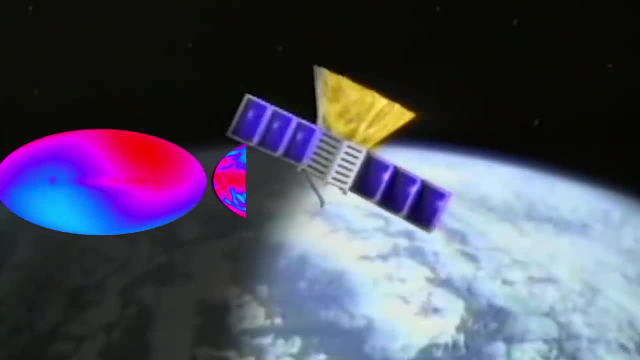 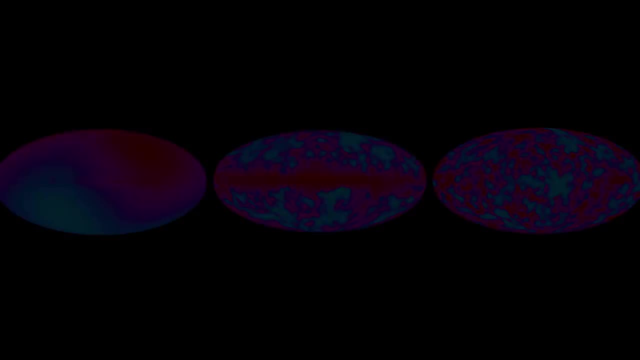 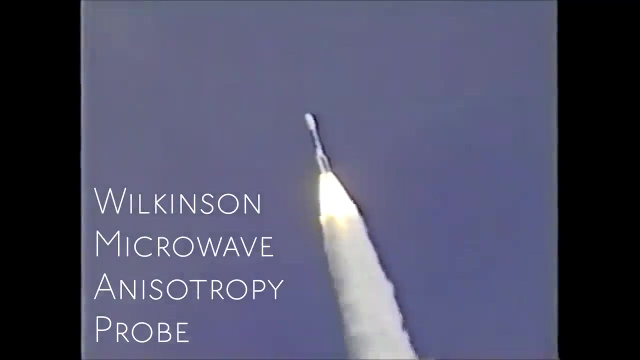 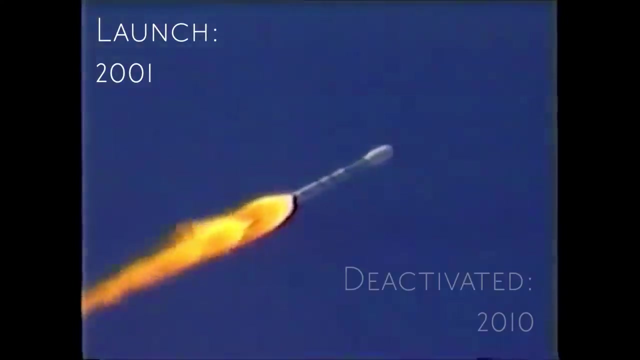 the equipment we have surveyed the CMB with since, but it nonetheless mapped large-scale anisotropies and gave us our first complete view of the whole universe at once. In the early 2000s, NASA launched the Wilkinson Microwave Anisotropy Probe, also known as WMAP. It launched in late June 2001 and ran up until 2010,. 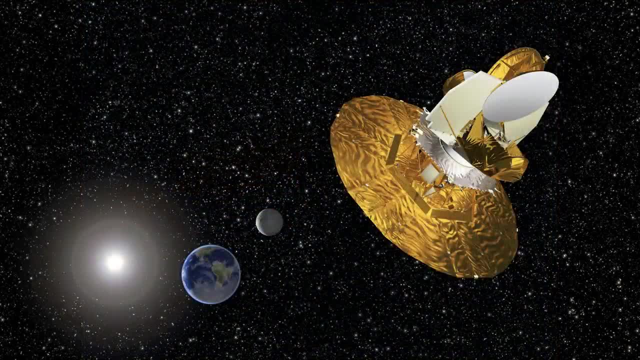 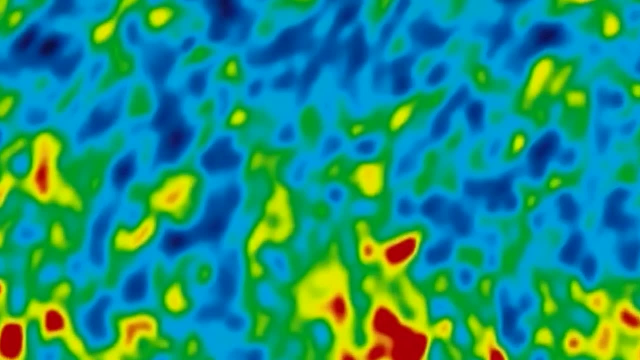 surveying the background radiation from more than 1.5 million kilometres away from the Earth. It gave us considerably more accurate and detailed measurements of the anisotropies and revealed heaps of new information about the age, size and structure of the universe. 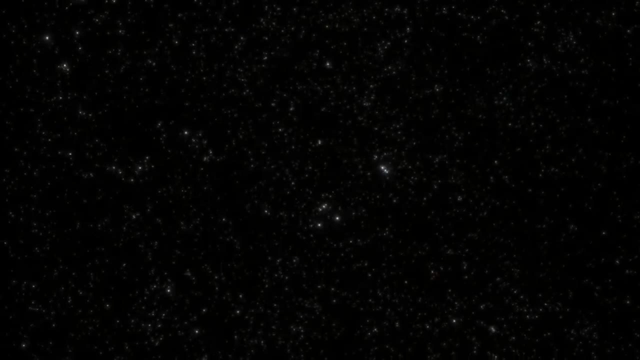 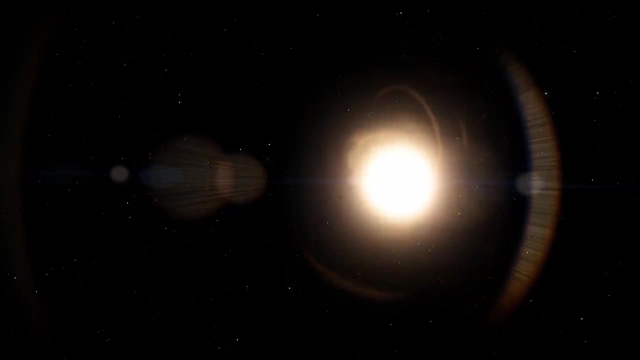 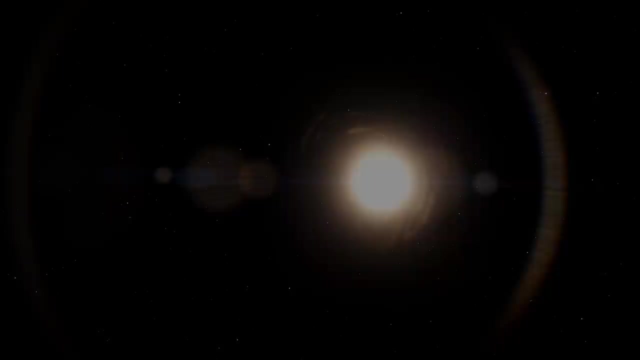 It revealed that the universe was about 13.7 billion years old, but that stars may have begun forming as early as 200 million years after the Big Bang- far earlier than anyone had predicted. And then, while the WMAP satellite was still active in 2009,, the European Space Agency 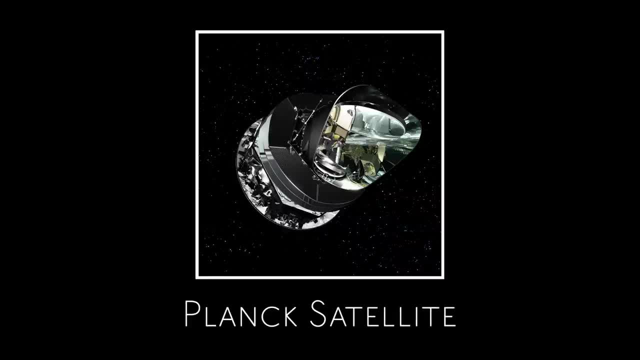 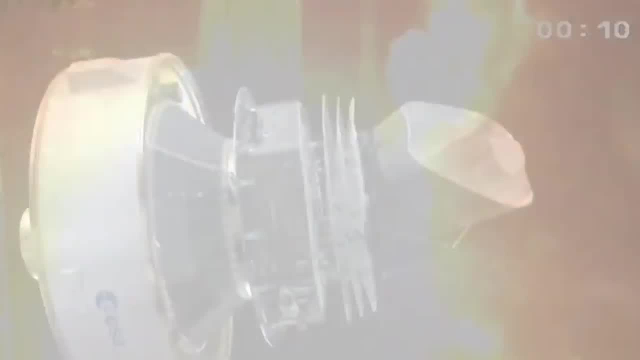 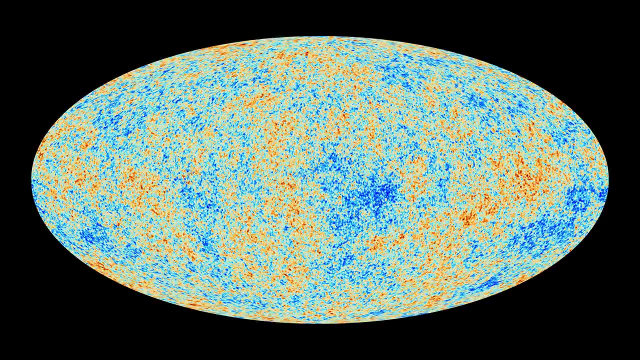 launched the Planck Satellite, By far the most sensitive and sophisticated mission to date. It was deactivated only four years after its launch, but this $700 million spacecraft nonetheless gave us our most precise, deep and complete look at the afterglow of the Big Bang. 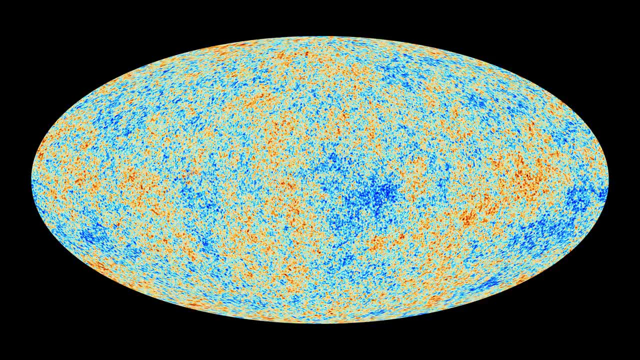 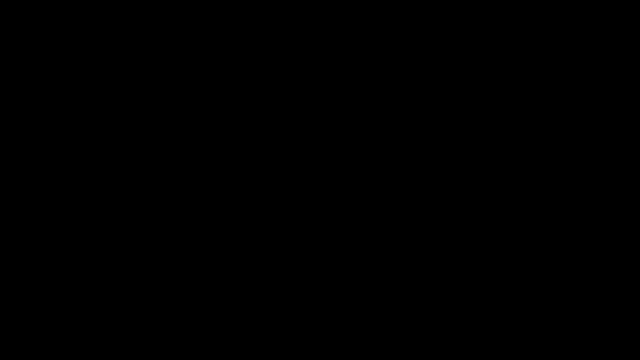 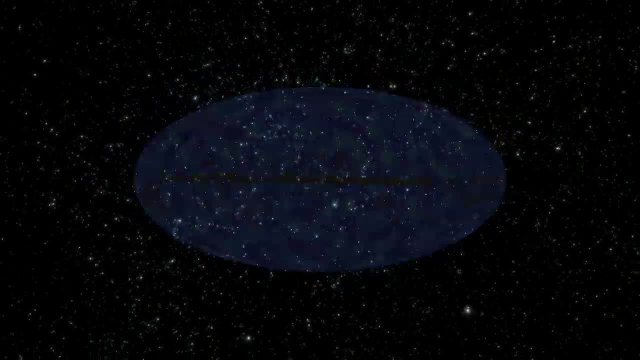 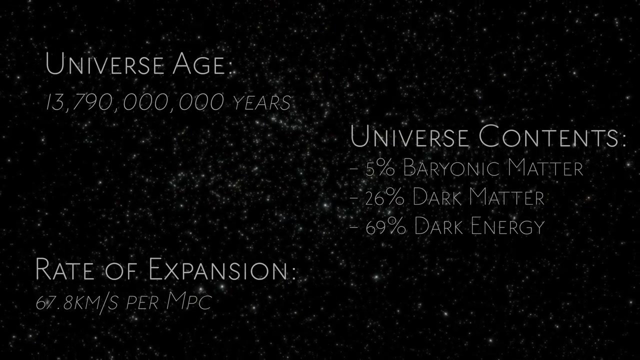 and it remains our most comprehensive snapshot of the early universe to date. The Planck Satellite gave us our most accurate measurements of the universe's age, its ratios of baryonic and dark matter and its rate of expansion. It recorded anisotropies on a scale three times more sensitive than WMAP and surveyed nine 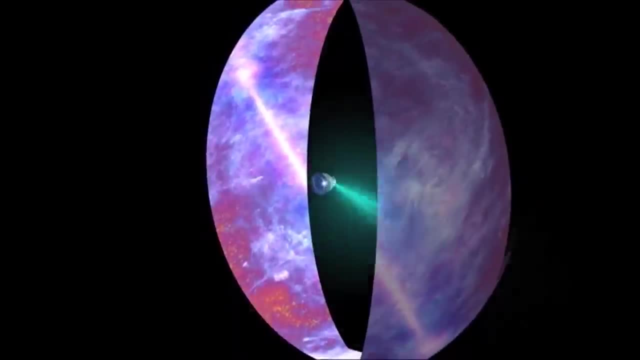 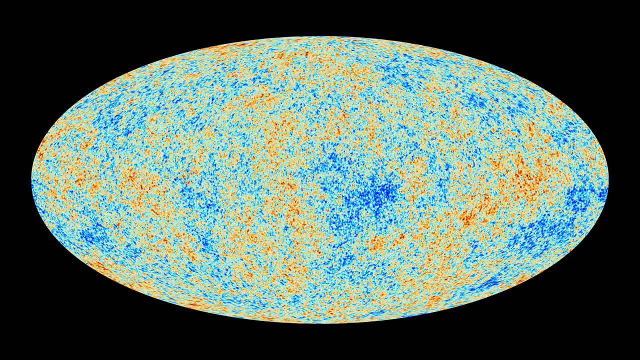 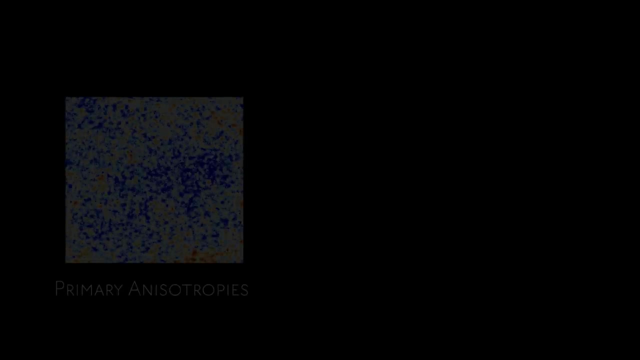 frequency bands in comparison to WMAP's five, enabling a much clearer and more concise view of the universe's anisotropies. So what exactly do these anisotropies do? Well, there are two main types of fluctuation- primary anisotropies, which are a direct result. 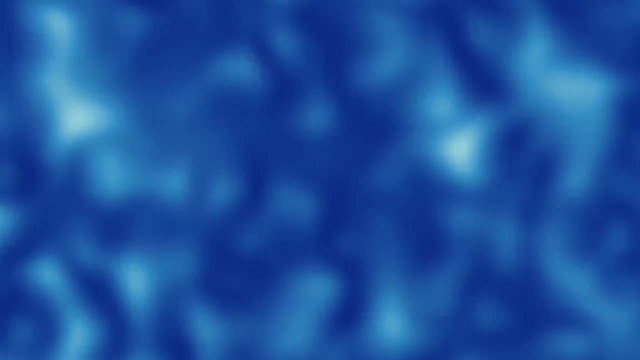 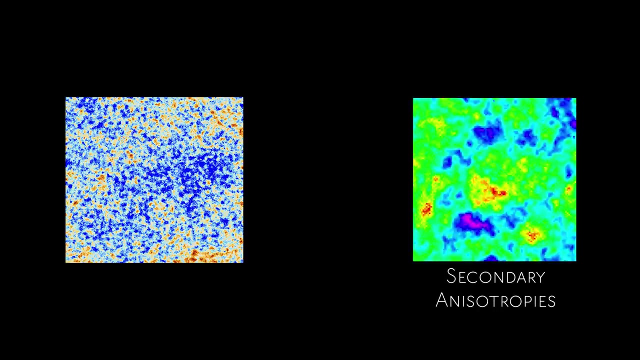 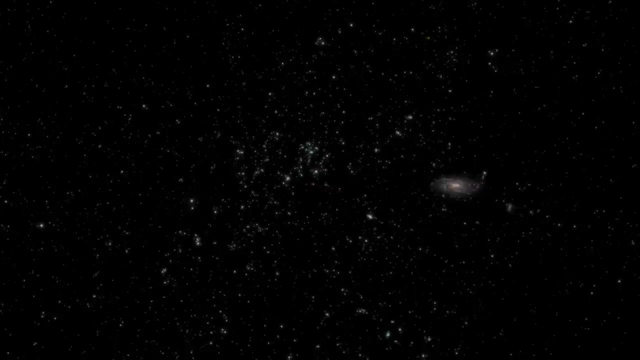 of the baryonic acoustic oscillation patterns frozen into the universe's plasma when it turned to atoms and secondary anisotropies, which are a result of stuff in the way of the CMB photons as they have travelled towards Earth like galaxies and voids. Therefore, this provides 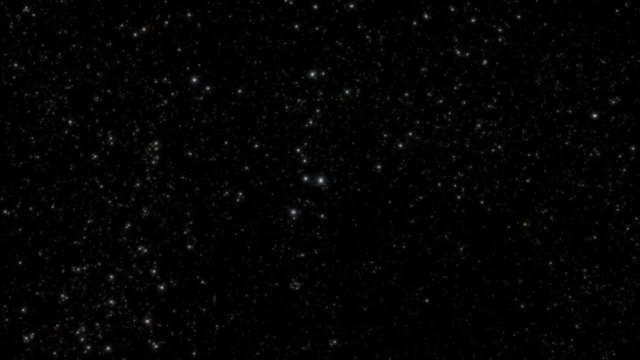 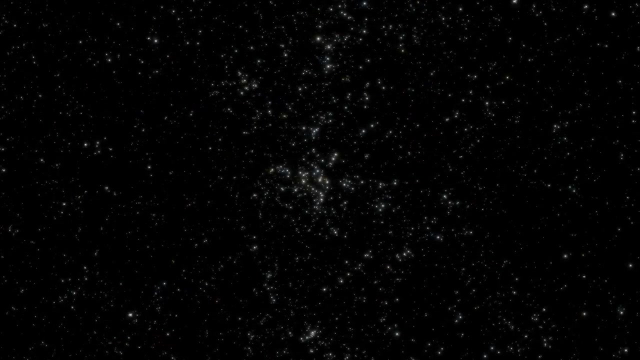 a great way for us to understand the universe's future and how it will change over time. So let's take a closer look at the universe's large-scale contents. Where we see red, warmer areas, we are looking at galaxies and galaxy clusters. 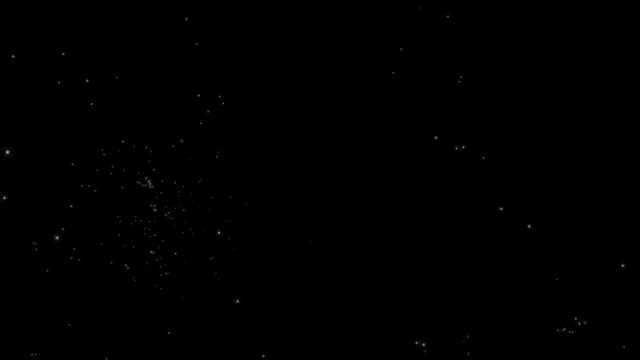 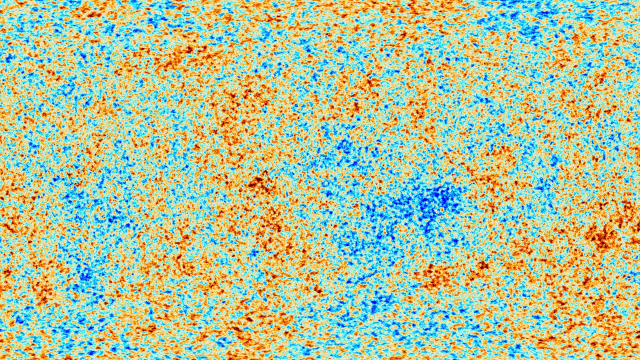 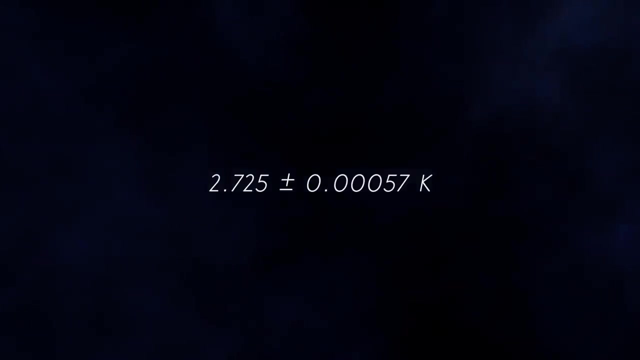 whereas the cooler blue areas correlate to voids and supervoids. The colours on the map do not represent absolute temperatures. rather, they show the level of deviation from the CMB's average temperature of 2.725 Kelvin. But, as we mentioned, 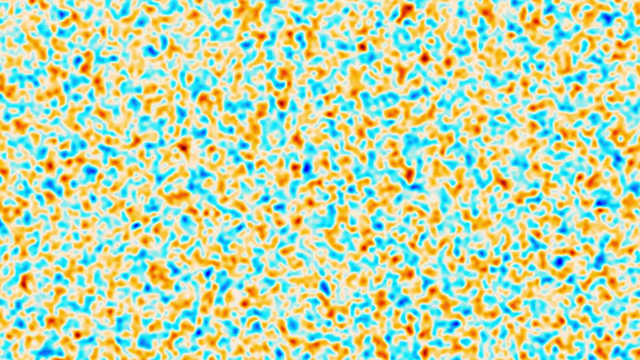 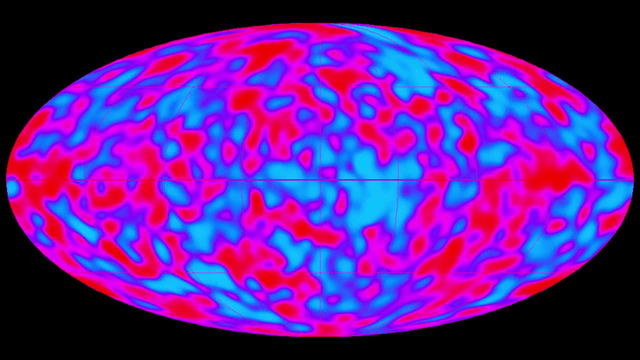 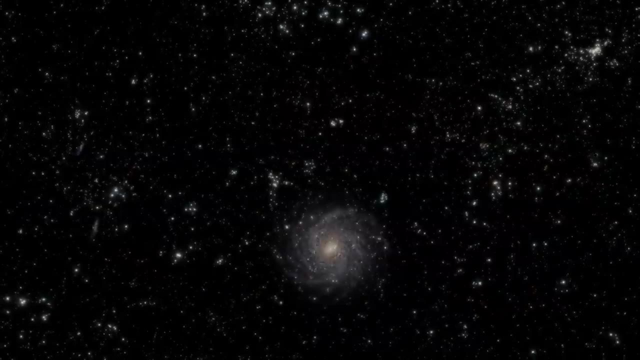 these deviations are on tiny scales of a few microkelvin- extremely marginal when compared with its absolute temperature. In a broad sense, the CMB shows us that the universe is smooth, isotropic and randomly distributed across its entire expanse. There are variations in gaps. 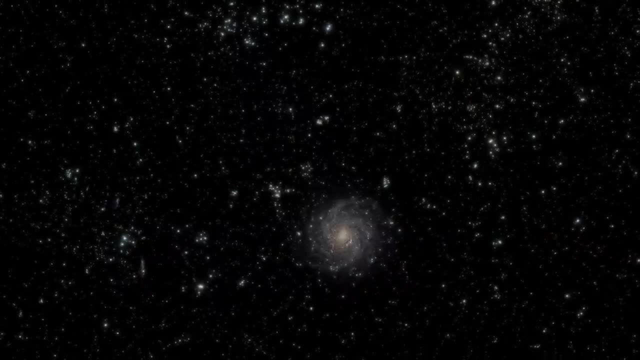 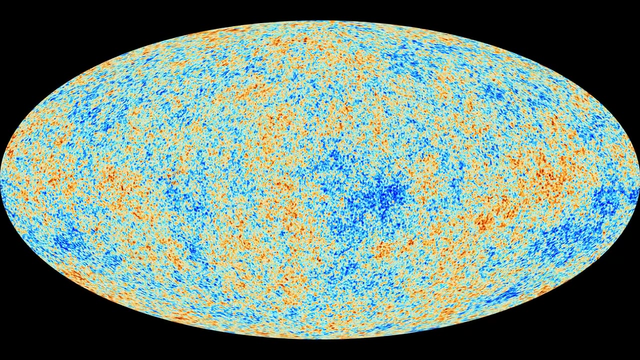 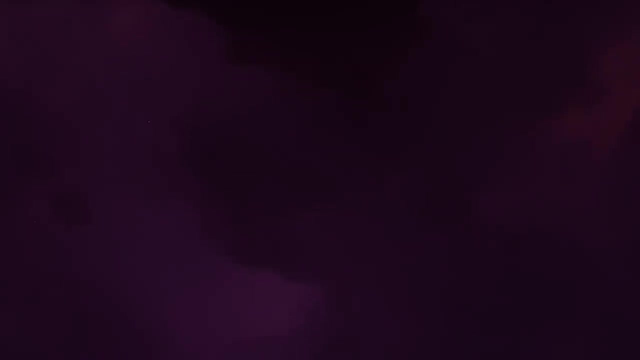 in space which are significant when compared with us, but when viewed on a wide enough scale, such as the CMB, these variations iron out To show a strikingly smooth cosmos, with its contents spread in a manner analogous to a homogenous hot gas. This informs and affirms one of our most fundamental yet controversial 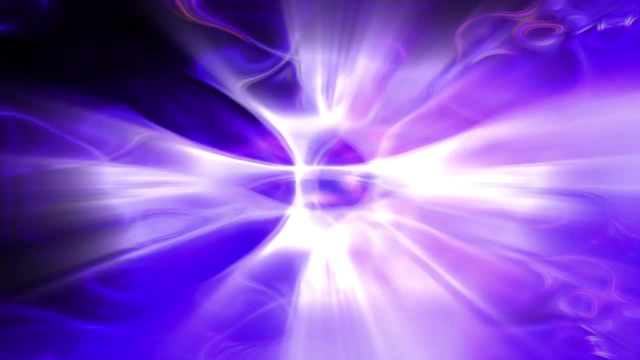 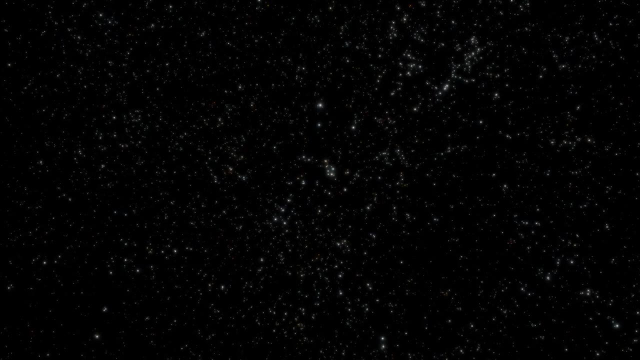 assumptions about the very early universe- the idea of cosmic inflation. In order for the universe to be so well distributed, even to this day, it must have been scaled up in size incredibly quickly and radically from the beginning. In the early years of the universe, the universe was a very, very 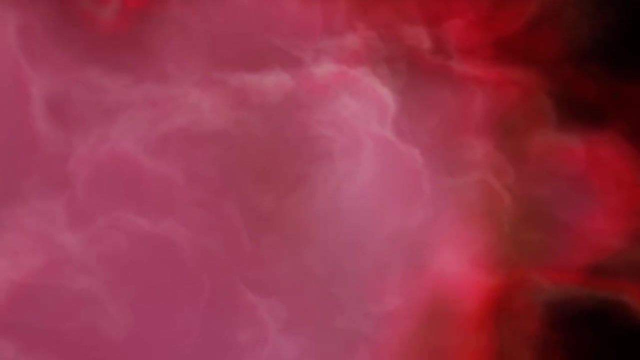 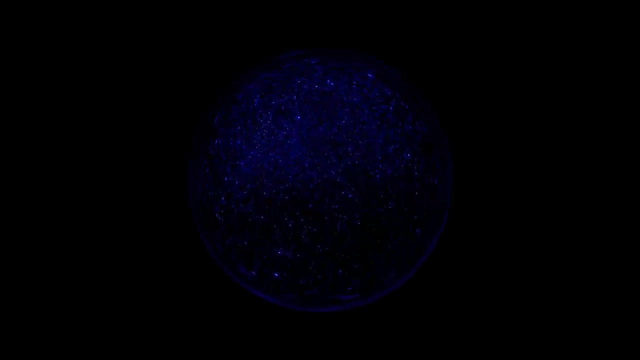 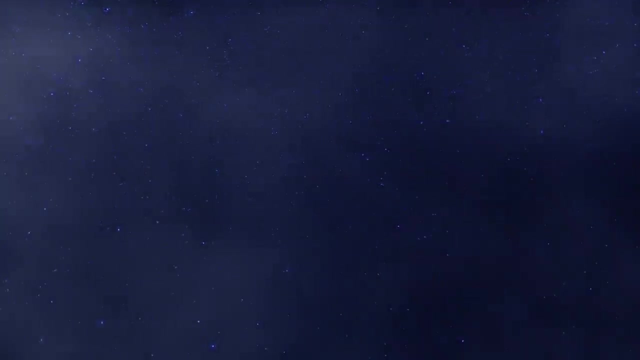 very small universe. The inflationary theory states that one of the earliest things to happen after the universe was born was an expansion event which appears to have violated all known speeds and laws in the universe today, Space was scaled up from nanometres to light years, all in less than 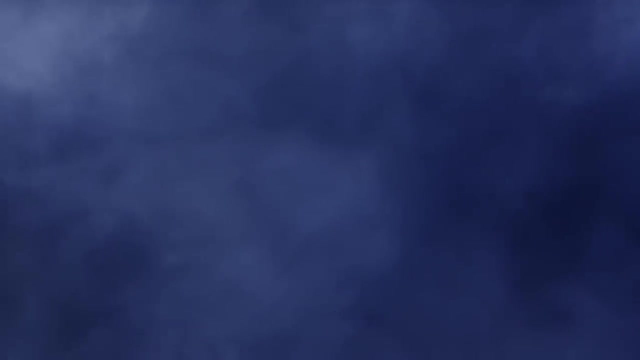 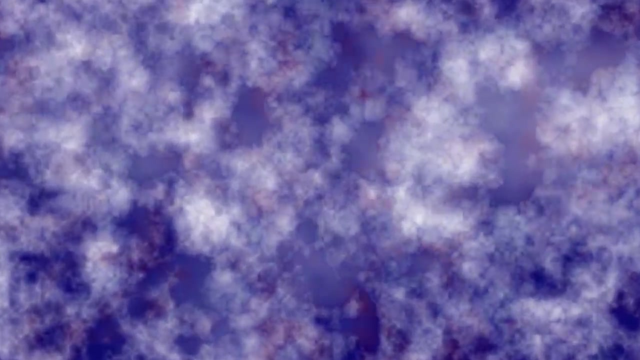 a microsecond. When this happened, the tiny irregularities and deviations in the very early universe's ultra-compressed contents were smoothed out and the universe was able to move out. The only fluctuations that remained were caused by small quantum ripples in the inflation. 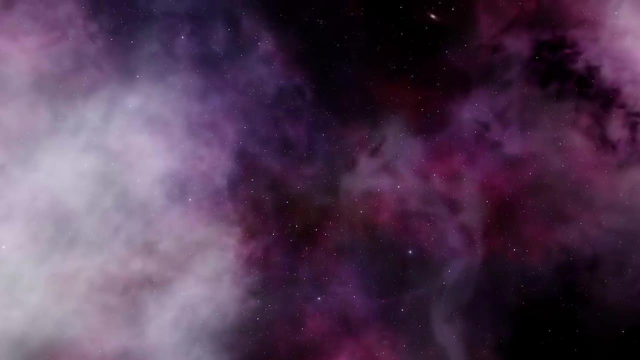 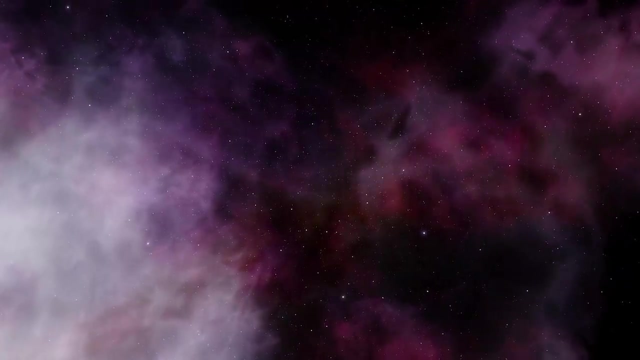 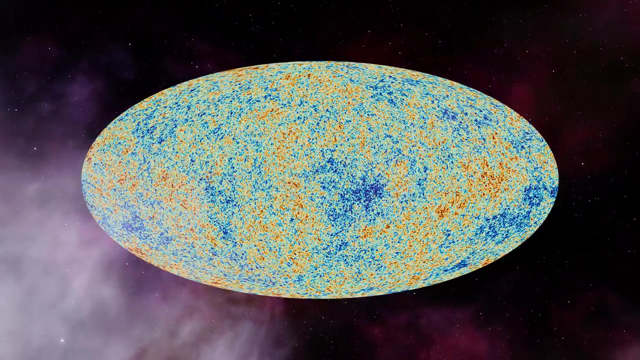 energy field, which gave rise to the minor variations that we see today. This theory has its fair share of sceptics, to be sure, and perhaps with good reason, But the remarkable uniformity of the CMB shows us that inflation fits the facts as well as any. 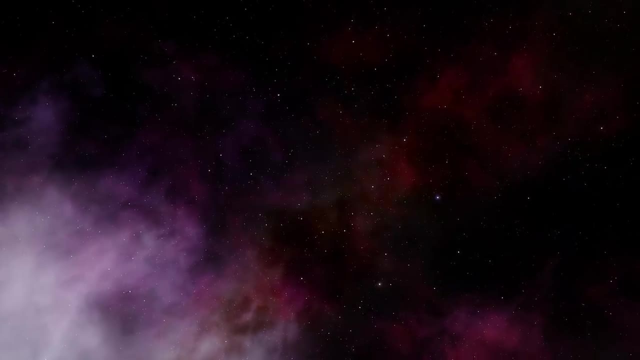 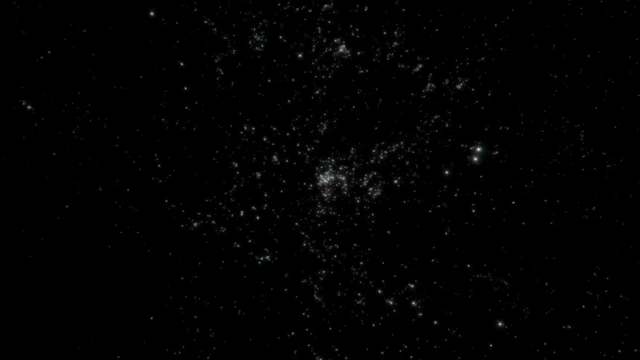 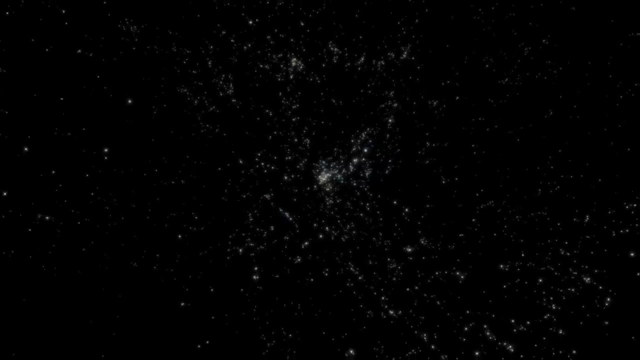 other alternative explanation. If the universe had grown any slower or in any other way, then gravity would have had more than enough time to distort the uniform structure of matter. No other theory can explain the CMB's origins and properties so precisely, and thus its existence lends a lot of credence to the Big Bang Theory. 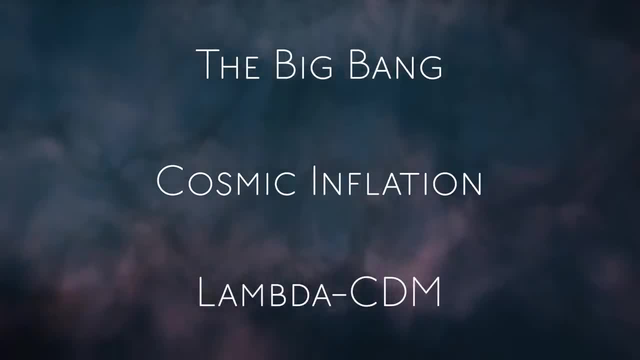 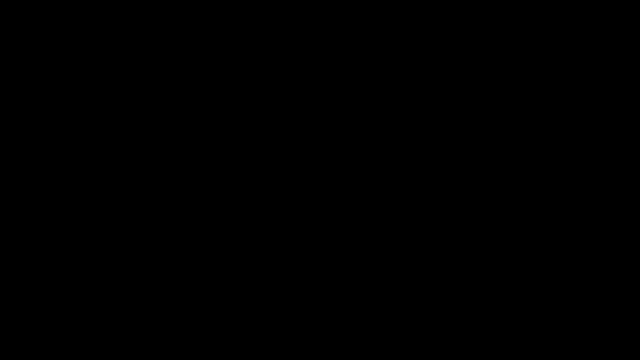 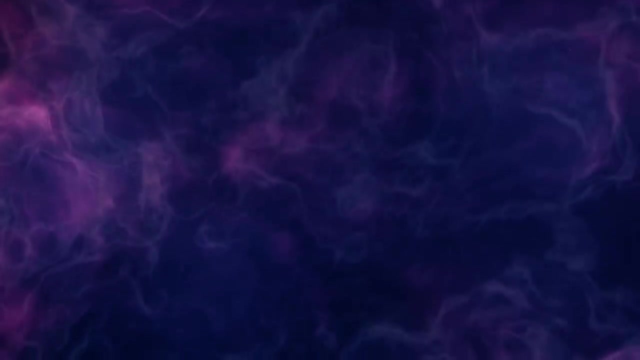 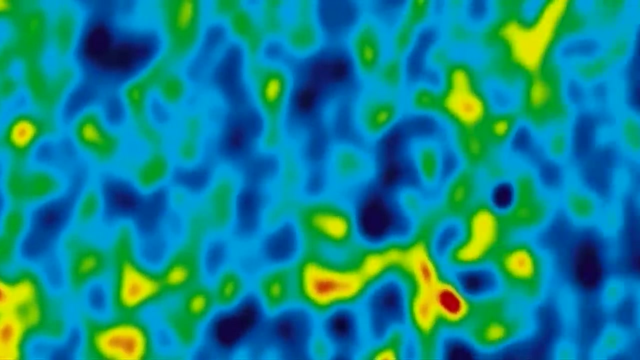 Cosmic Inflation and the Lambda-Cold Dark Matter model overall. So that's the story of the Cosmic Microwave Background and of our universe And, like with any great discovery in cosmology, there exist anomalies and unanswered questions within the CMB which we still can't account for. Specifically, anomalously warm and cold. 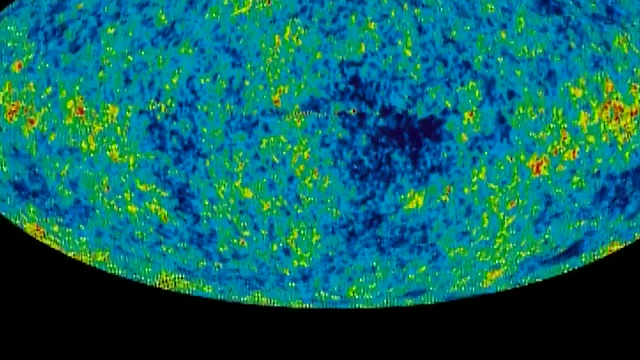 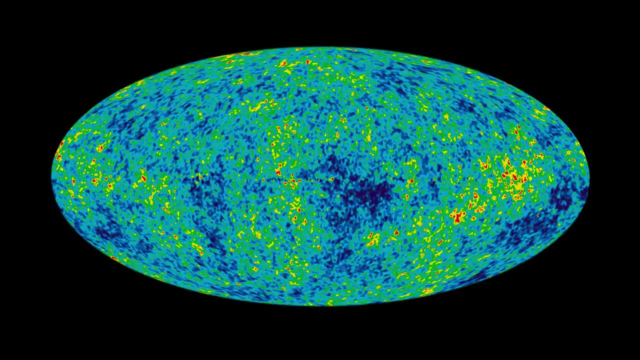 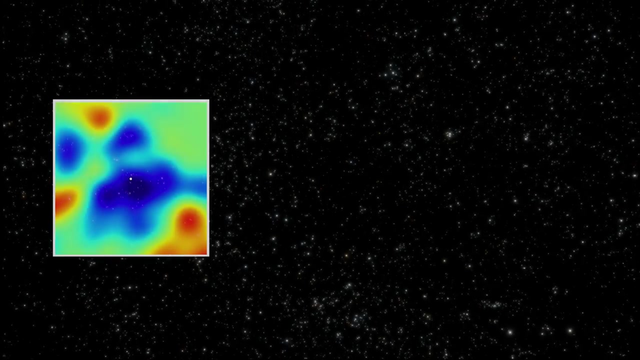 areas of the radiation which seem unnatural when compared with the near uniformity of the microwave sky. Let's start with the latter, An unusually large and cold anisotropy in the Southern Galactic Hemisphere, aptly known as the Cold Spot. The Cold Spot is an area of the CMB where the temperature drops very sharply when compared. 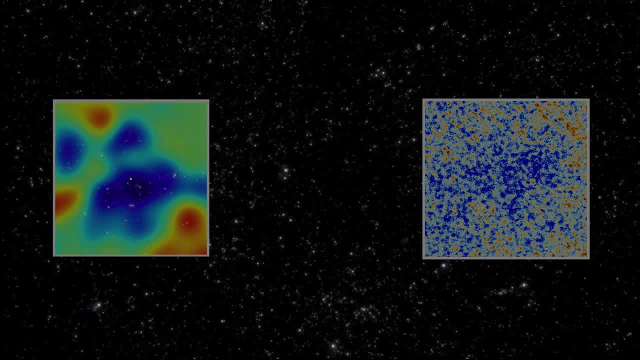 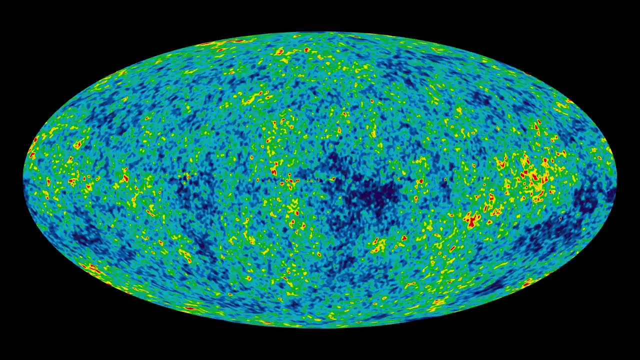 with other anisotropies, implying that there is something more at work than simply a less dense region of space. This anomaly was first noted by the WMAPS satellite before being unexpectedly detected again by the Planck Satellite, which is also known as the Plank satellite affecting the CMB's temperature drop. This is a 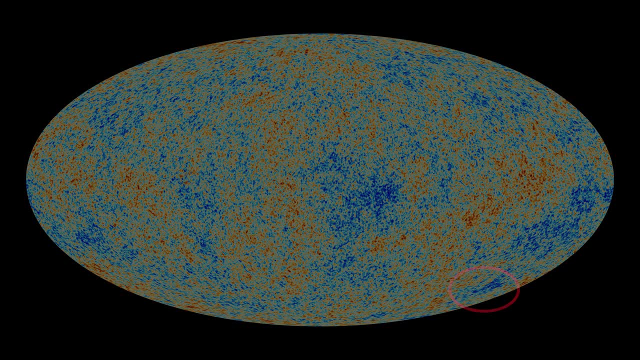 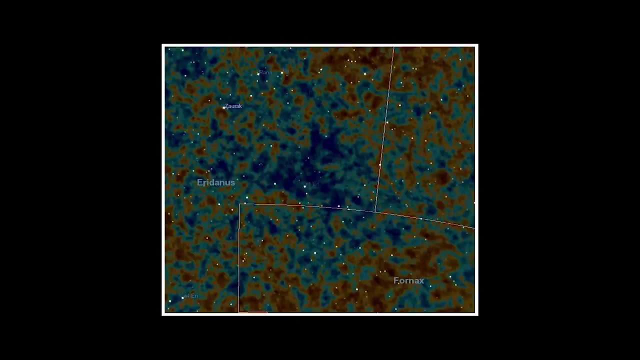 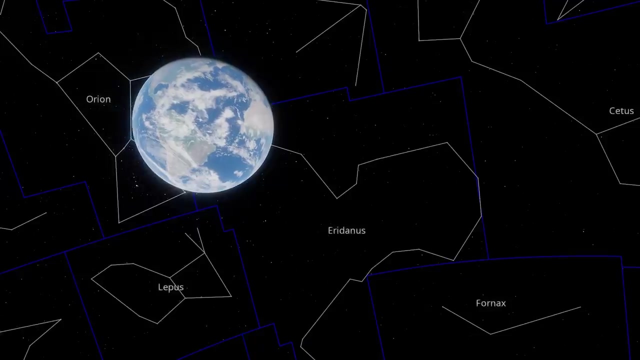 effectively ruling out the possibility of it being a data processing error. Whatever, the cold spot is, this thing actually exists somewhere out there in the darkness. The anomaly is located predominantly within the constellation of Eridonus and has a width in the night sky of more than 20 times the diameter of the Earth's moon. 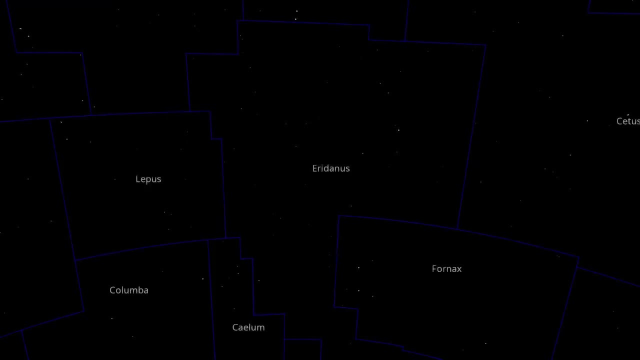 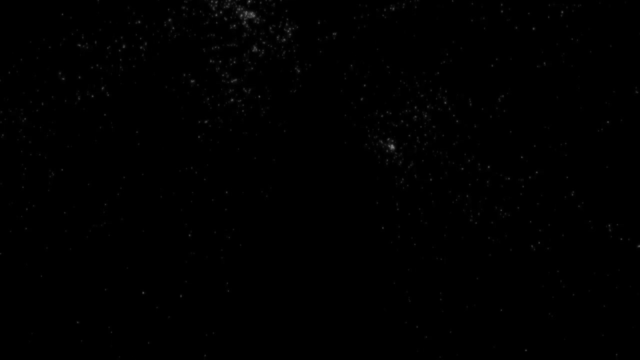 correlating to a cold, empty patch of space hundreds of millions or perhaps even billions of light-years wide, making it one of the largest things in the known universe. It is several times larger than the average size of cold anisotropies and while 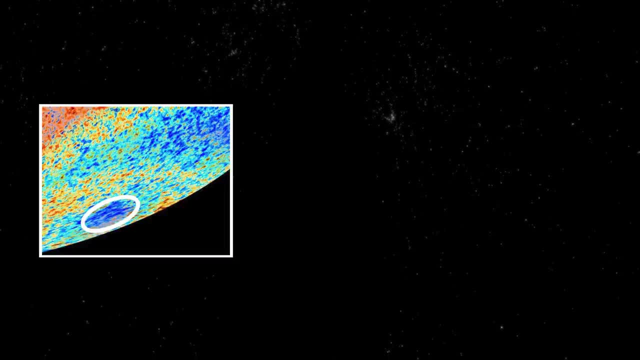 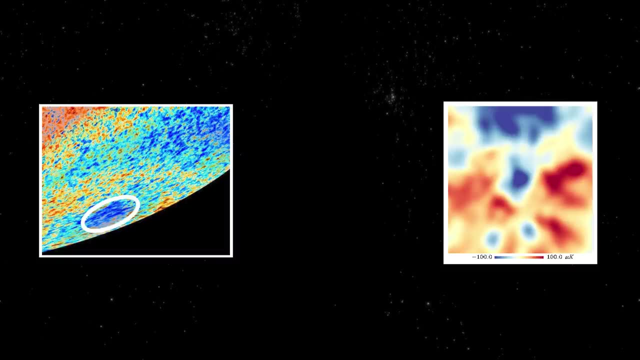 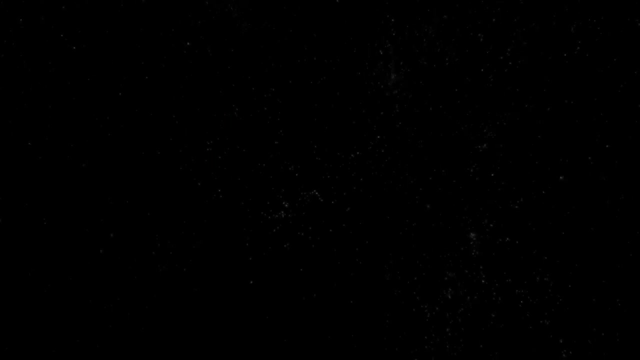 average temperature fluctuations within the CMB are around 18 microkelvin. the cold spot dips by an average of 70 microkelvin and in some places it drops by more than 140 microkelvin. Voids and supervoids can usually explain such large cold areas, because voids have a diminishing 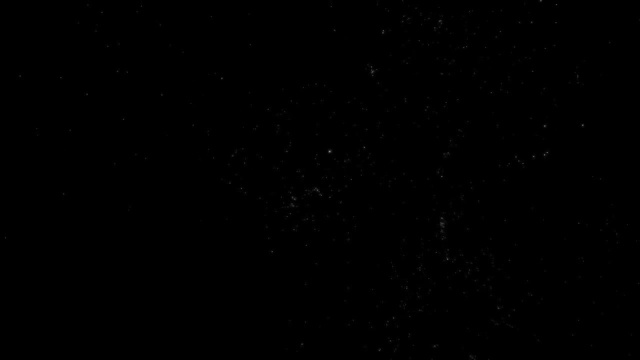 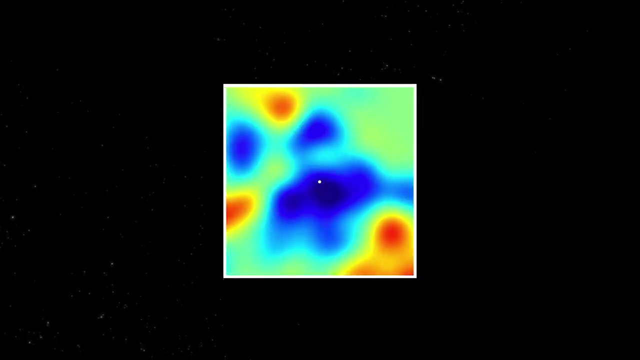 effect on the energy of the photons travelling through them, including the CMB photons. But even the light-sapping effect of a void of this enormous, unlikely size would not be sufficient to account for the sharp drop in temperature that we're seeing. In fact, some scientists argue that Big Bang, cosmology and the idea of a smooth 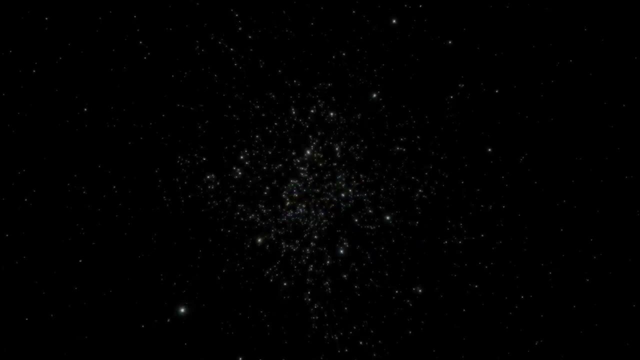 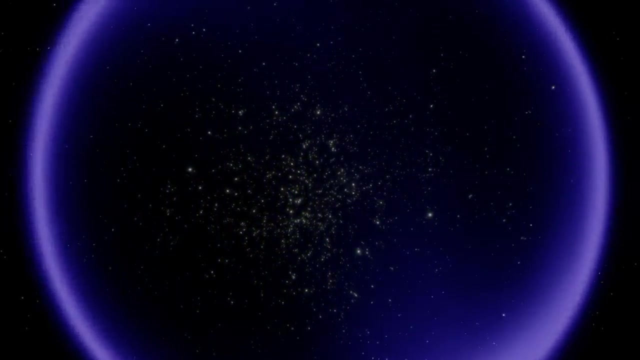 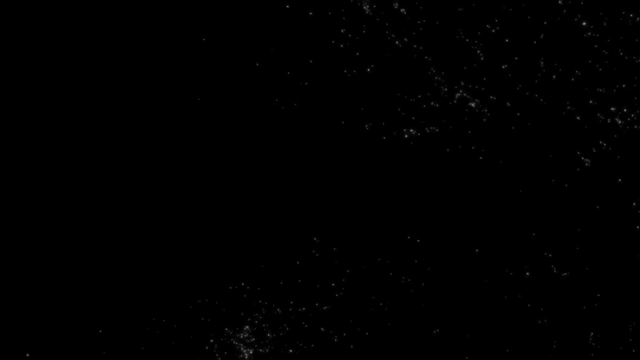 isotropic cosmos cannot account for such a large anomaly period. If the universe really is nearly homogenous by the grace of cosmic inflation, then such a universe should not be able to naturally give rise to such a large, empty and cold supervoid. And so naturally the inexplicable. 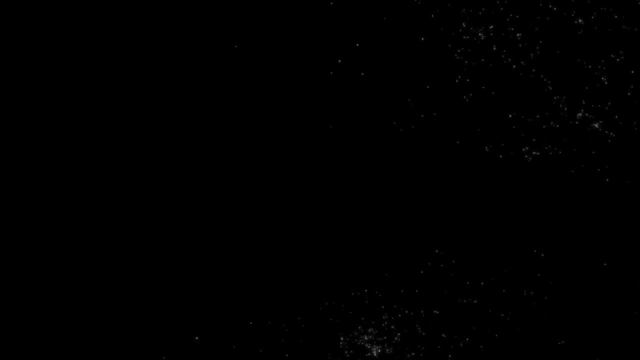 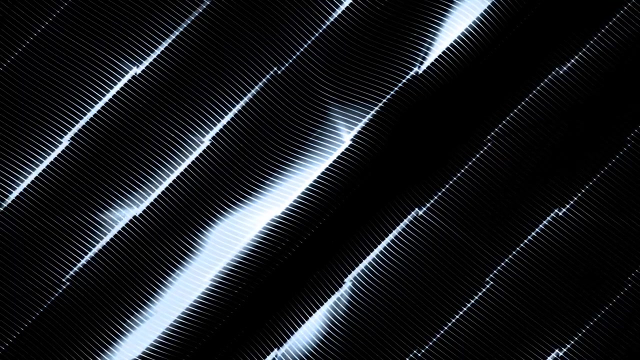 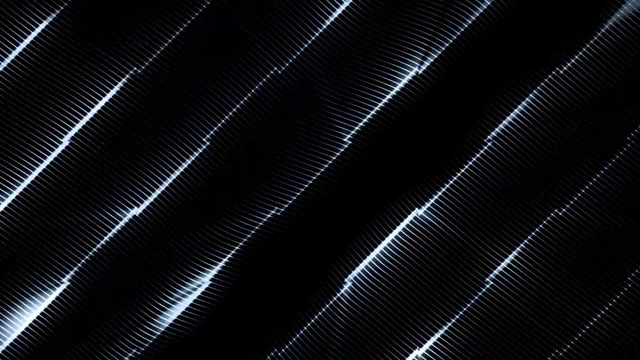 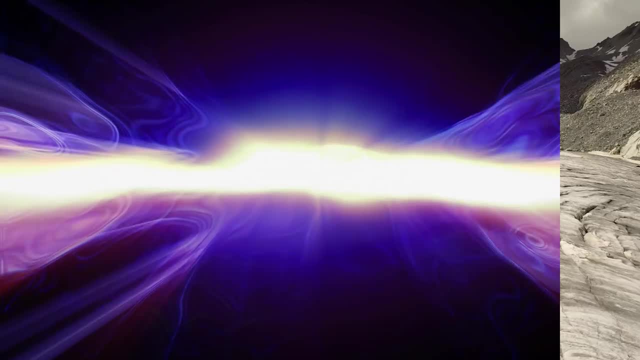 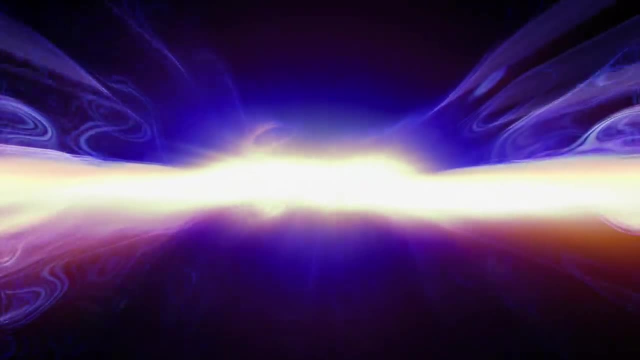 a damaged or defective area of the universe, analogous to a crack within an ice sheet. No known physical mechanism could allow for such a defect in space, and thus cosmic textures are hypothetical at best. But some have taken this a step further, claiming that the source is extra. 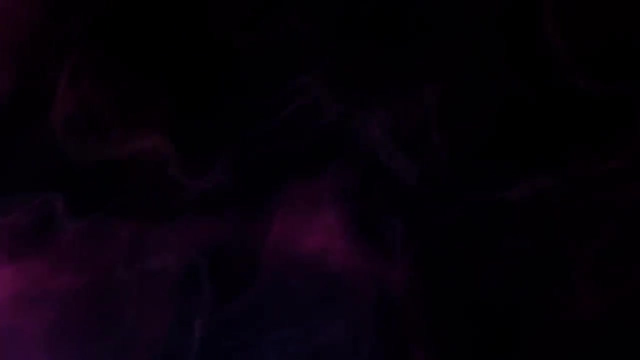 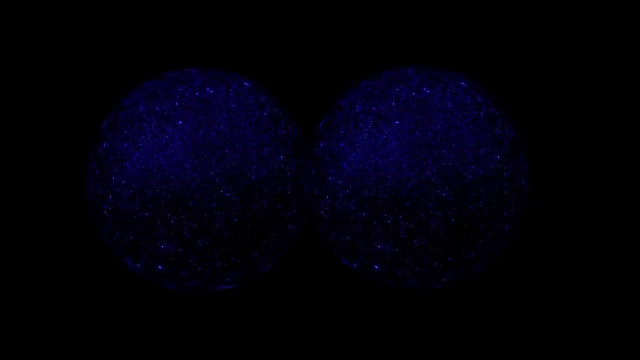 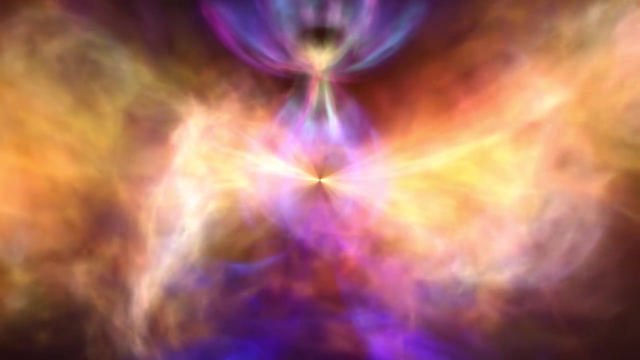 universal. Some propose that the cold spot is a bruise from where our universe bumped into another bubble universe, while others propose that the cold spot is an imprint from where our universe became quantumly entangled with a perfect parallel when it sprung into existence, before the two were. 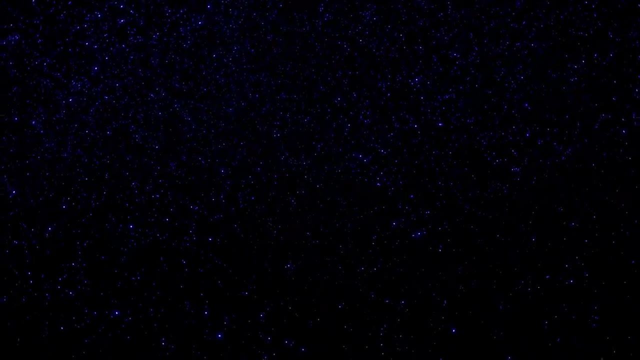 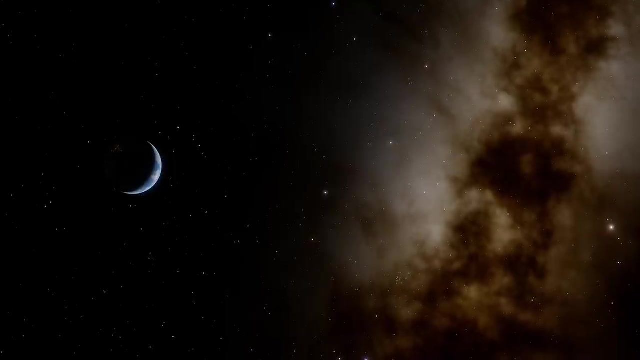 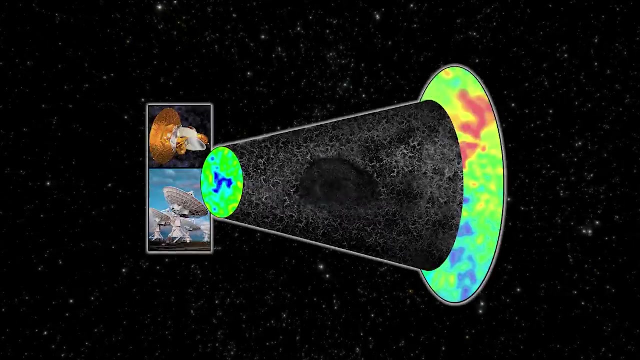 separated by cosmic inflation, But those are admittedly some pretty outlandish and, at the moment, unevidenced hypotheses. While it is an intriguing mystery and a spooky coincidence, the cold spot is more than likely going to be due to some kind of improbably large void, perhaps with the help of a few data processing artifacts, or 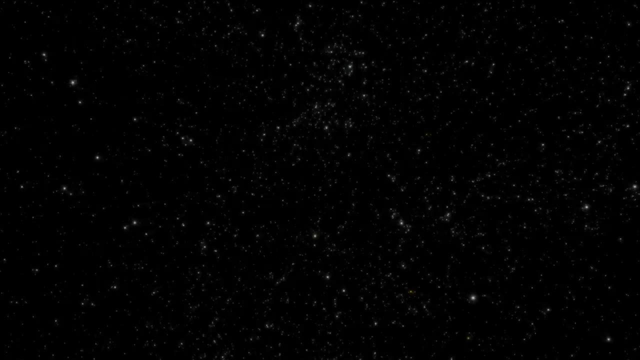 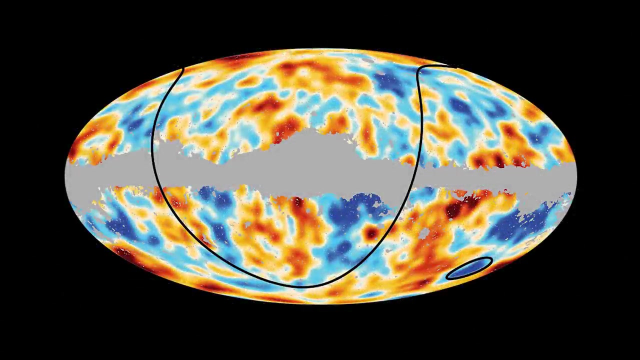 something in the way to enhance the effect, Or Cam's razor and all that. But don't get too disappointed, because the cold spot is not the only anomaly on the CMB which might imply some kind of alternate reality. And in contrast to the cold spot, these anomalies constitute 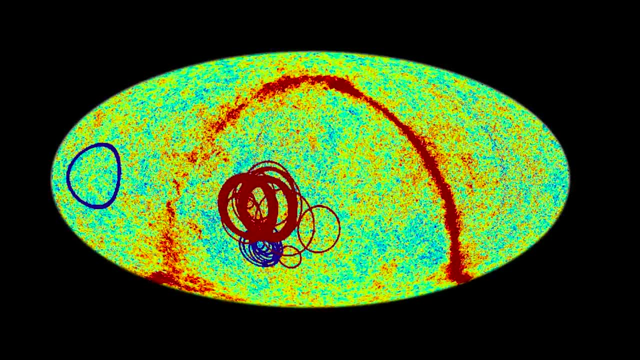 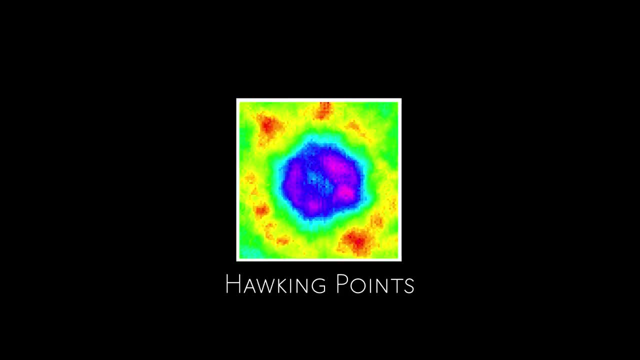 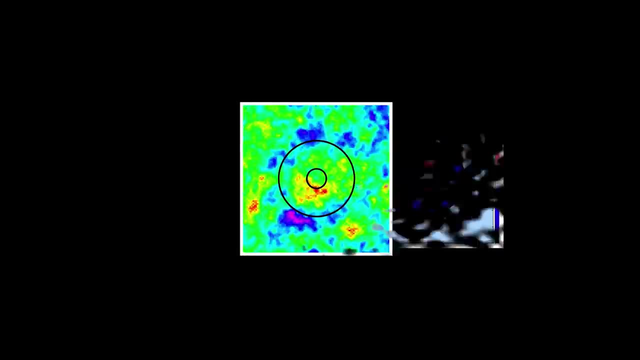 significantly warmer than average regions, as opposed to cold ones. I'm talking about Hawking Points- powerful spherical sources of energy within the CMB- around 8 times the diameter of the full moon. Within these spots, the temperature fluctuates sharply upwards by more than 30 times the mean temperature increase for warm anisotropies. 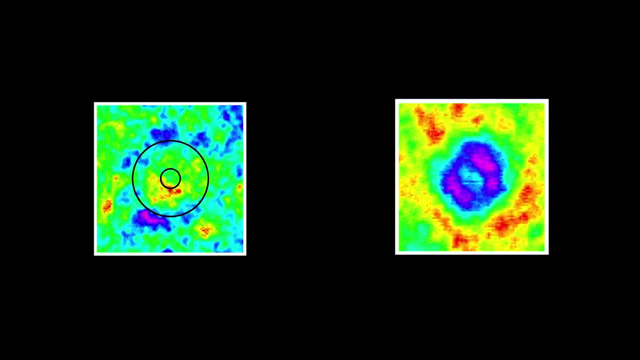 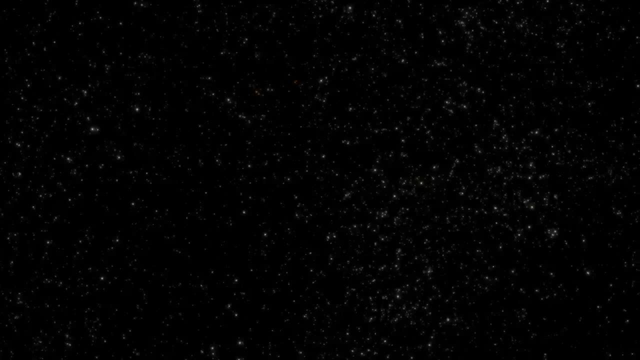 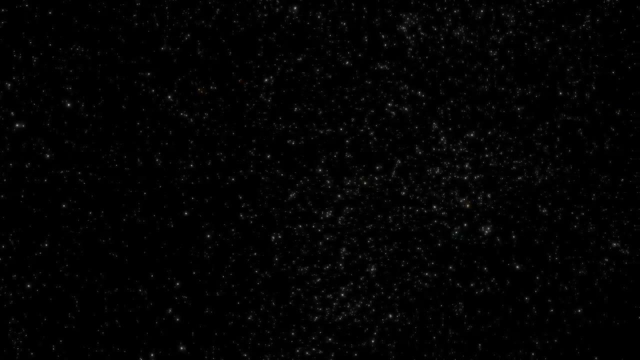 suggesting that they are sources of high amounts of photon energy. These points went undetected for the longest time- it was assumed that any anomaly like this would be an artefact of data processing, as cosmic inflation wouldn't allow for such irregularities. But after being noticed on the Planck Satellite data, these points were 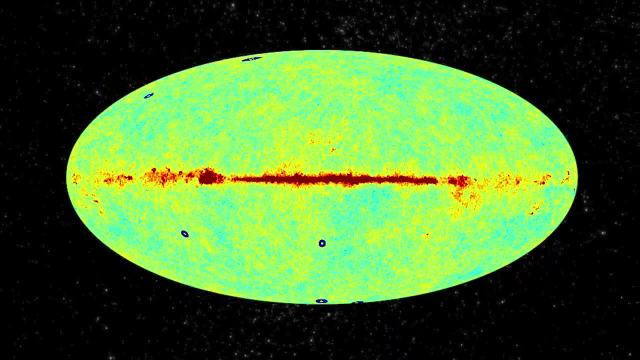 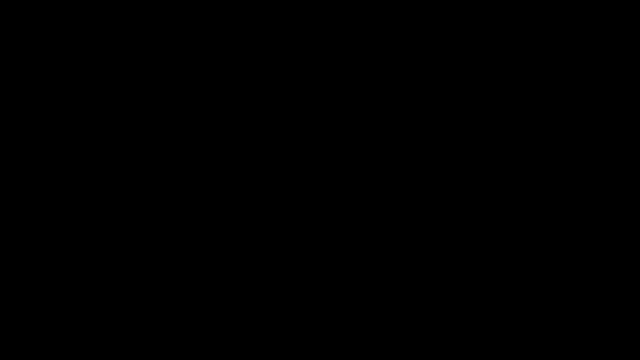 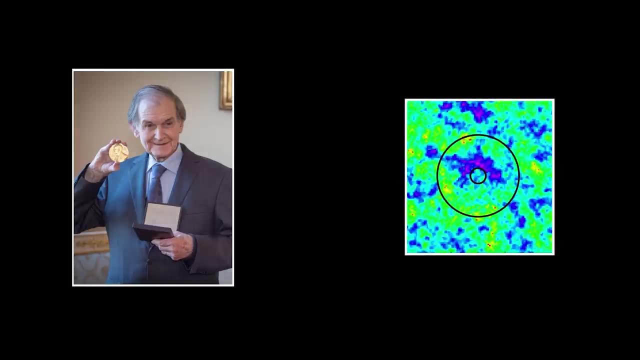 then confirmed within the WMAP data as well. Analysis has since revealed no less than 30 of these points within the CMB, and some scientists, in particular Oxford mathematician Roger Penrose, believe that these points are in fact echoes from a previous iteration. 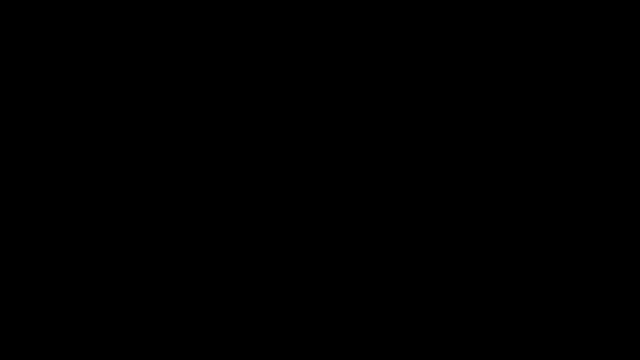 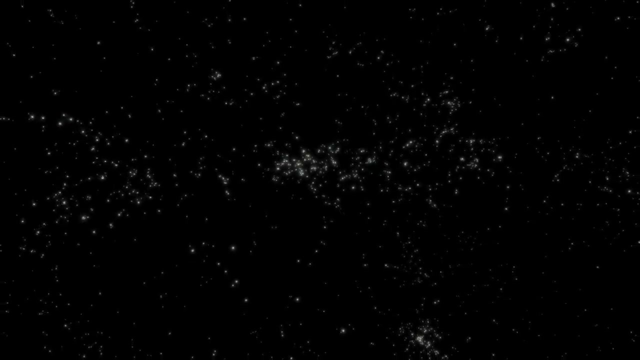 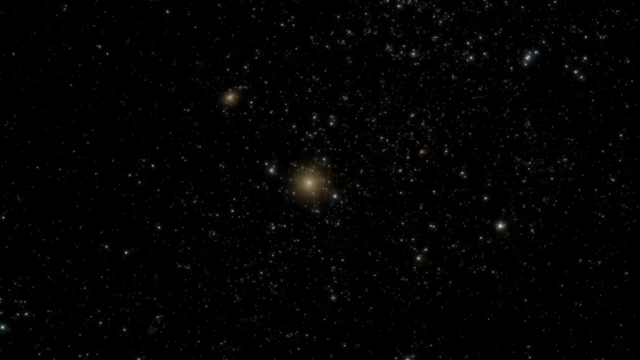 To understand why one must consider an alternative twist on the Big Bang theory, namely the paradigm of conformal cyclic cosmology, which proposes that our universe is just one in a number of so-called aeons or cycles of our universe being born, expanding. 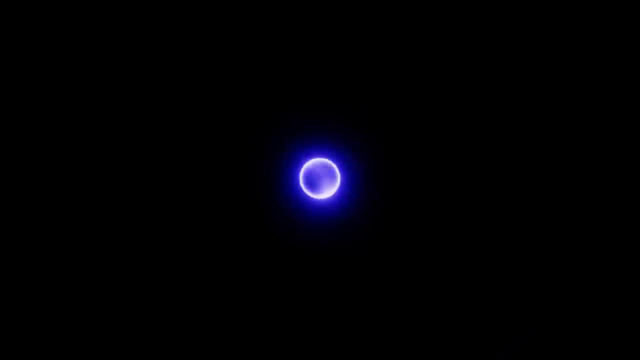 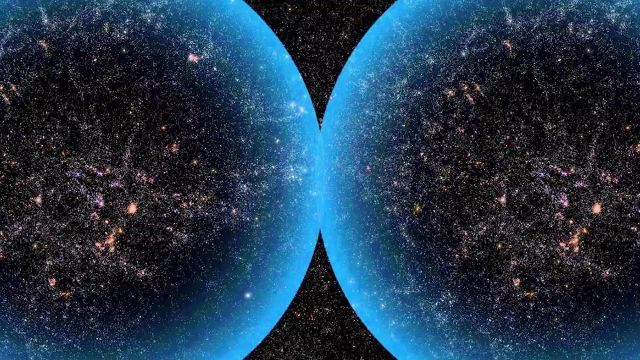 and then collapsing down into a new Big Bang to be born again, with the process repeating at infinitum. Not a parallel universe, like what's being suggested with the cold spot, but rather an oscillatory universe which expands up and then squashes down repeatedly. 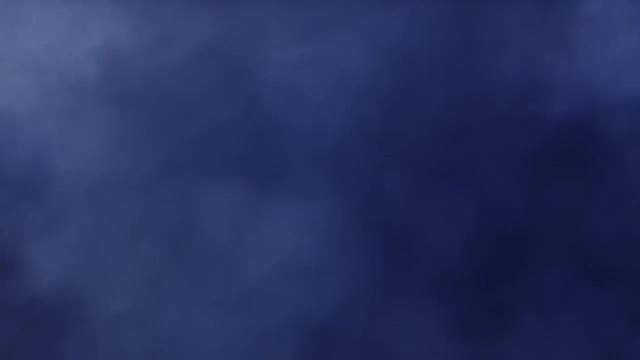 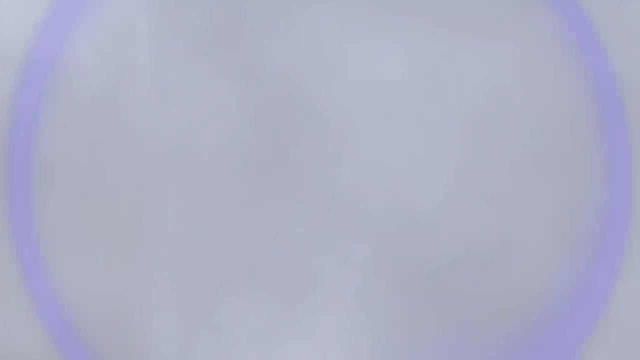 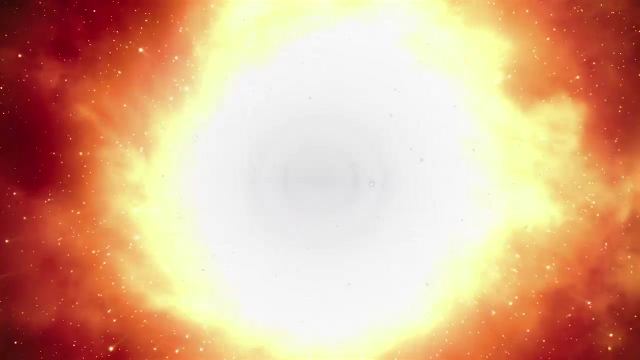 One of the major selling points of conformal cyclic cosmology is that it offers a slightly more explainable hypothesis for cosmic inflation, moving it to before the Big Bang of our universe. The theory suggests that what we perceive as cosmic inflation in the nanoseconds after the Big Bang was actually the very remote and far future of. 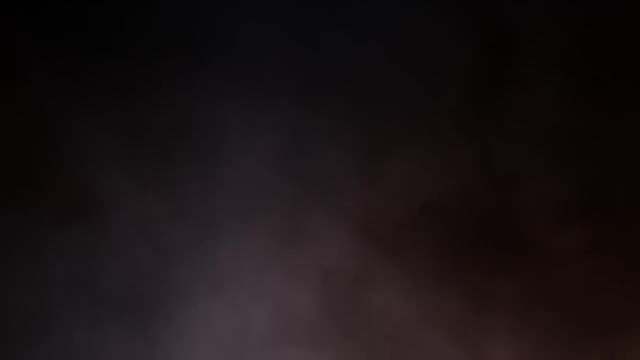 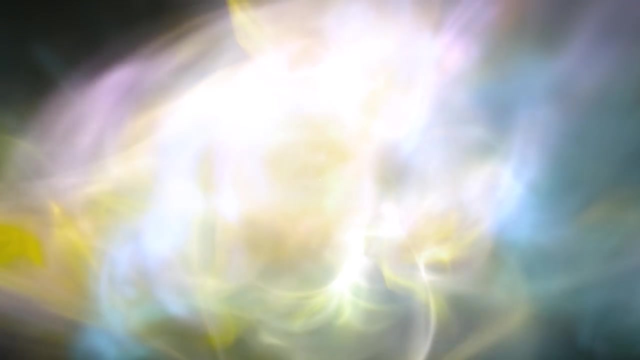 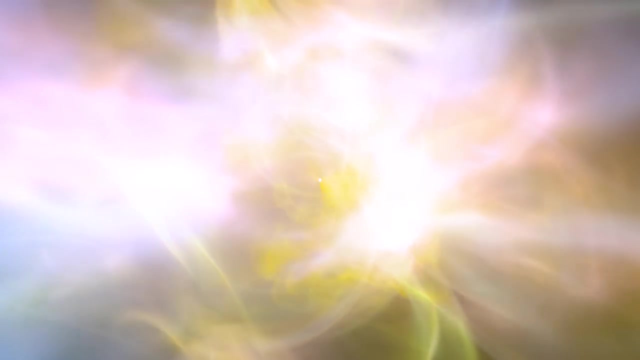 the previous universe, which was so old and vast and expanding so rapidly that it mimicked the behaviour of what we believe happened during the inflationary epoch of our universe. So where does the CMB come into all of this? Well, conformal cyclic cosmology proposes that during the previous universe's rescaling event, 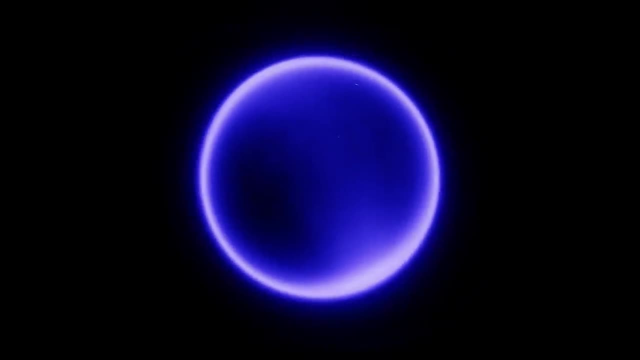 when it is squashed back into the big bang. it will be a time of collapse, where it will be a moment of loss or collapse, or collapse into a new Big Bang. the only thing that will exist by then are black holes, which will 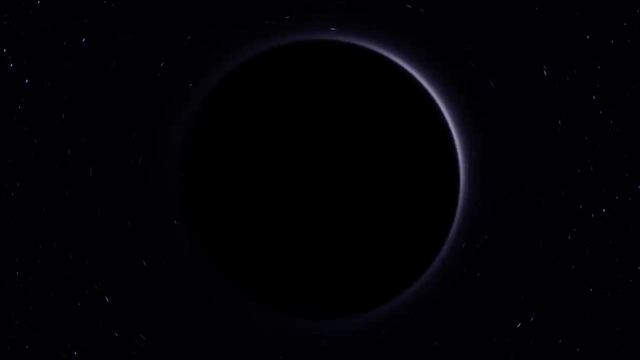 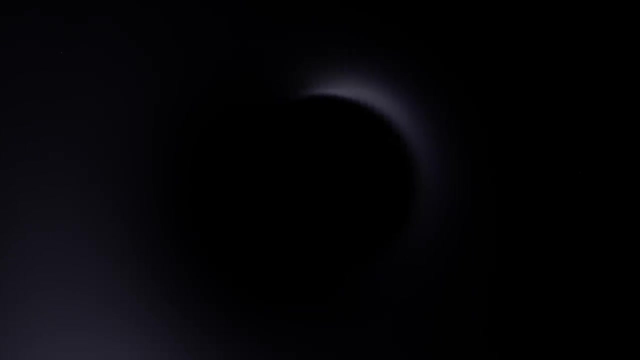 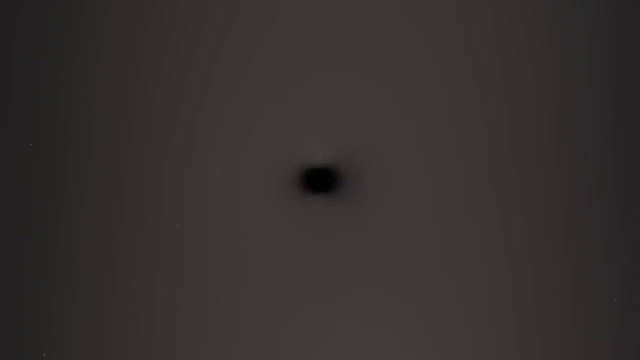 have had more than enough time in their remote futures to consume their entire galaxy groups and each other, leading to a few unfathomably massive black holes dotted around the enormous universe. But this exponential expansion in the previous universe's future occurs at near-timelike. 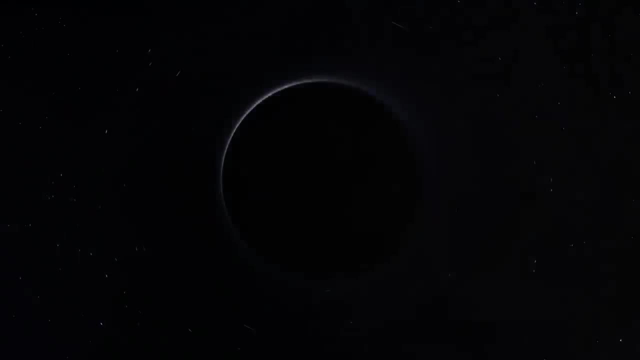 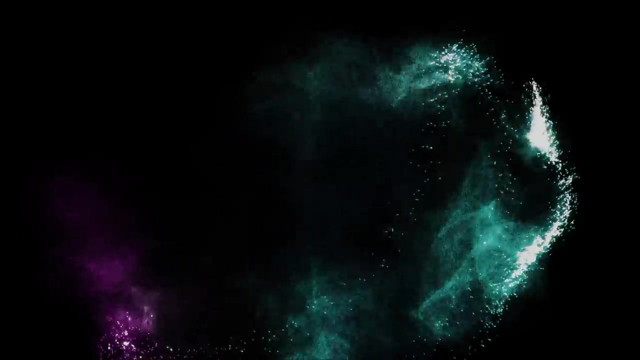 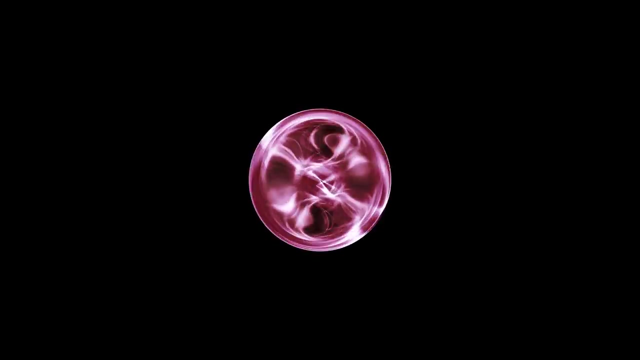 infinity, long after even the largest black holes will have evaporated into Hawking Radiation. The Hawking Radiation is what will then be squashed back into the new Big Bang, but rather than being blended in with the new universe's contents, this energy is retained as a single. 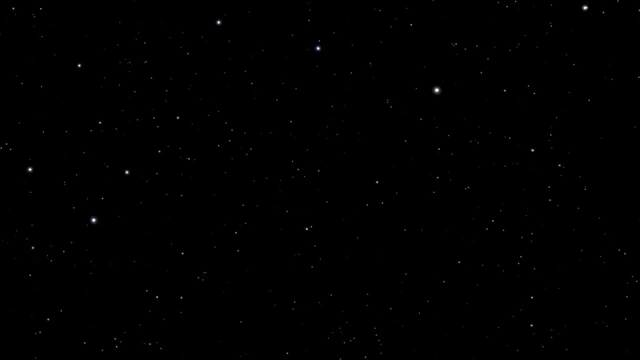 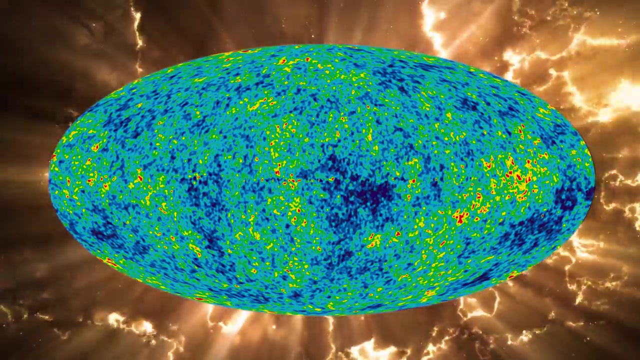 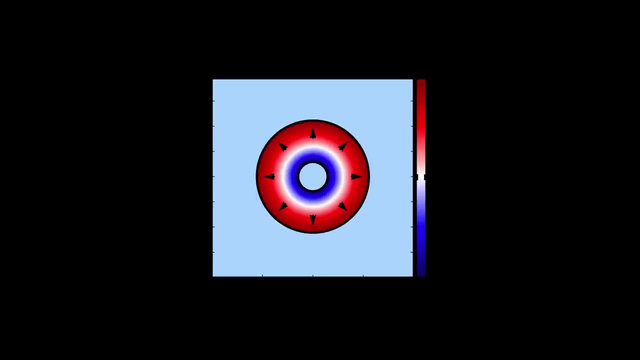 point which persists into the new iteration. It is only during the new universe's epoch of recombination, when it's CMB which is created, that this photon energy is freed. And if all this is true, then by now any such point in the preceding universe should. 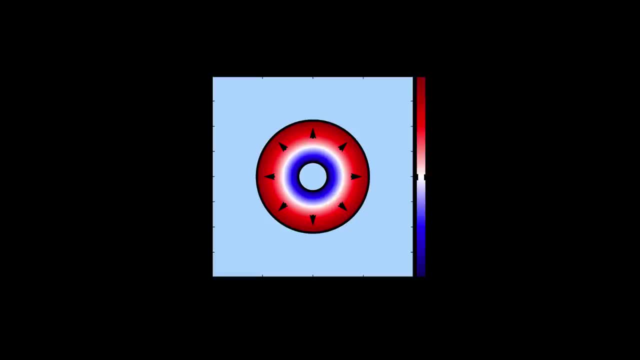 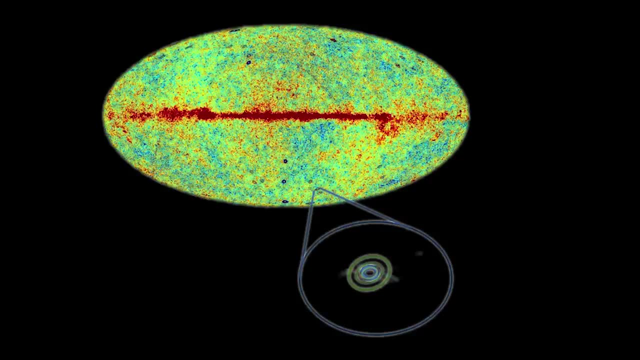 be about 3 or 4 degrees of the sky, across around 8 times the diameter of the full moon. And sure enough, this is what has been seen in the CMB data and proposed by Penrose et al as evidence of an oscillatory universe. 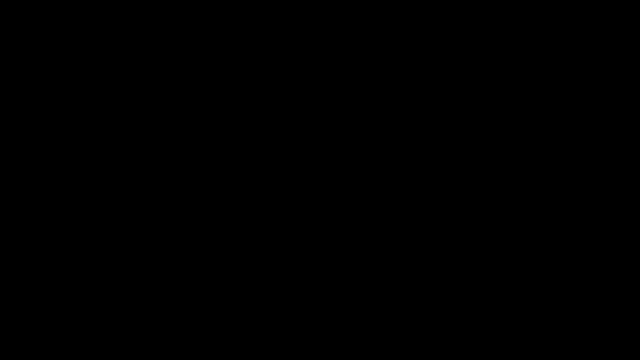 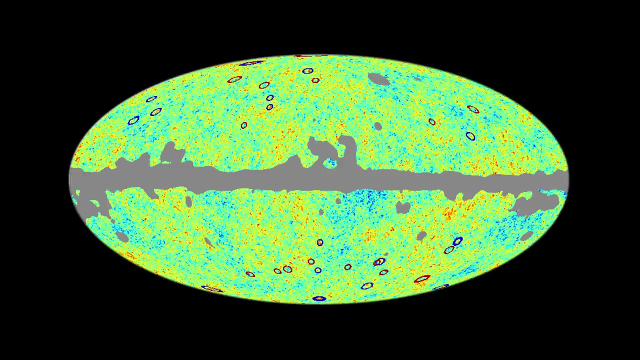 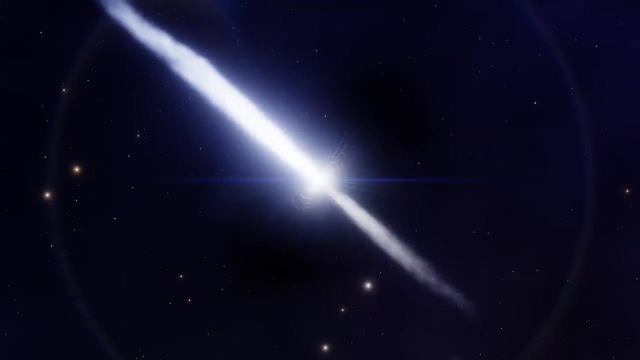 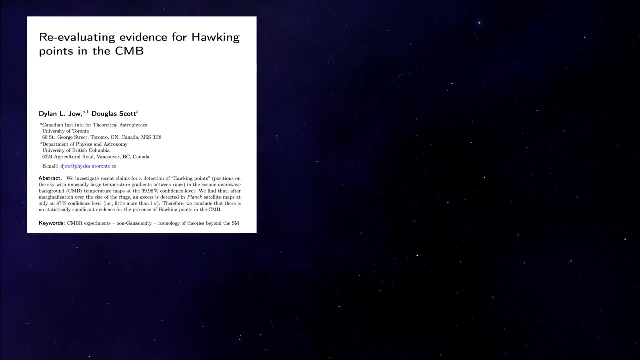 Pretty spooky right. There are no less than 30 of these points lurking within the CMB map. The question is: are they really the evaporated ghosts of 30 massive monster black holes from a previous universe? Not everybody thinks so. Follow-up studies have suggested that the findings for Hawking points are not as statistically 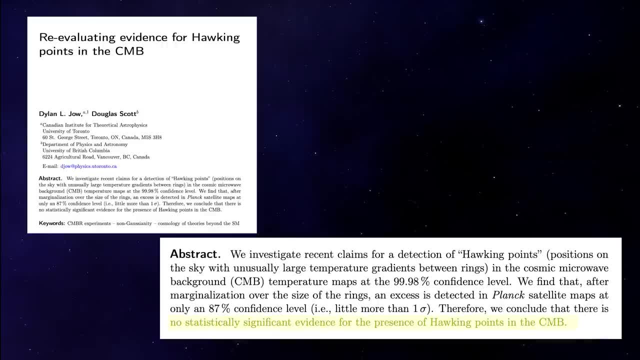 significant as they were first thought to be. In summary, the Hawking points are not as statistically significant as they were first thought to be. The Hawking points are not as statistically significant as they were first thought to be. In summary, the jury is still out on the nature of Hawking points, as it is for the nature